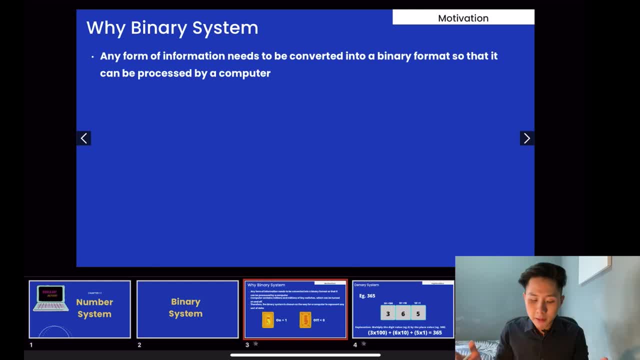 they need to be converted into a binary format so that it can be eventually processed by a computer, Which means binary is the only language which a computer can speak in. And this is because computer contains millions and millions of tiny switches which can be turned on and off. 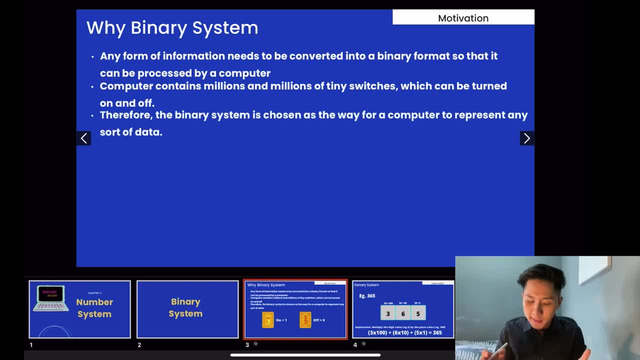 So let me explain. Therefore, binary system is chosen as the way for a computer to represent any sort of data, in which, when we turn on the switch, it means the value 1.. And when we turn off the switch, it represents the value 0.. 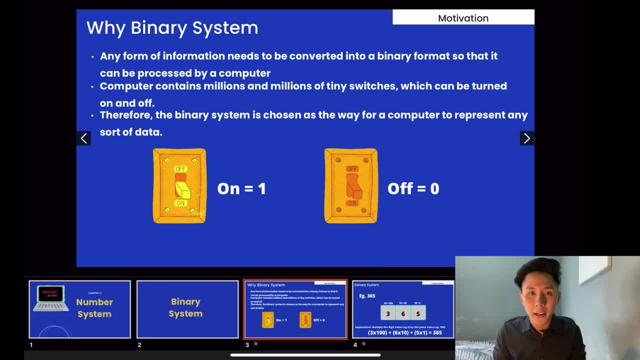 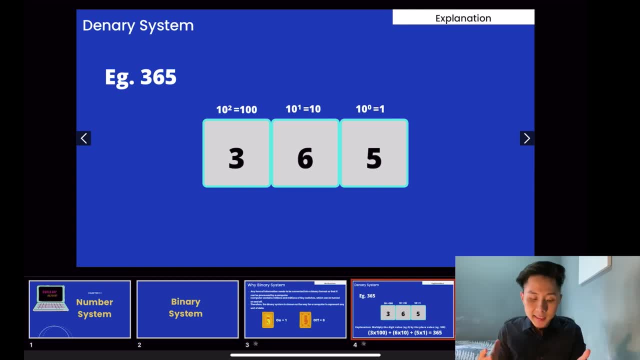 Therefore, in binary system there are only two possible values: 0 and 1.. But think about it, The basic system that we use in our day-to-day life. for instance, we have 365, the number of days in a year. 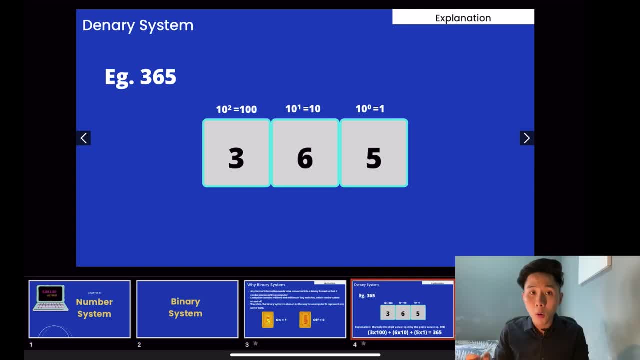 The number system that we are used to is called the binary system, In which we know that this value is 365 by multiplying the digit value, let's say 3, with the place value 100.. So we will do 3 multiplied by 100. 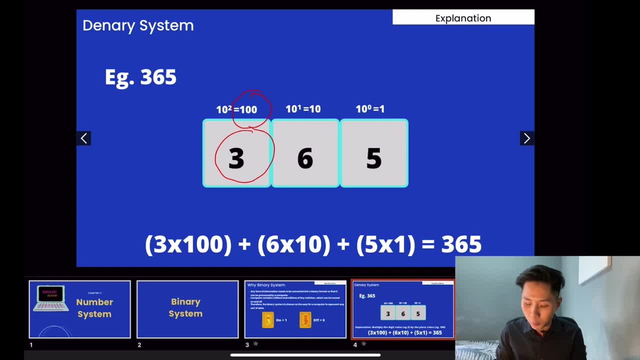 6 multiplied by 3.. 6 multiplied by 10.. 4 multiplied by 1., And eventually we got the value 365.. And yes, this is how we understand numbers in our day-to-day life. But, as I mentioned, computer cannot understand binary. 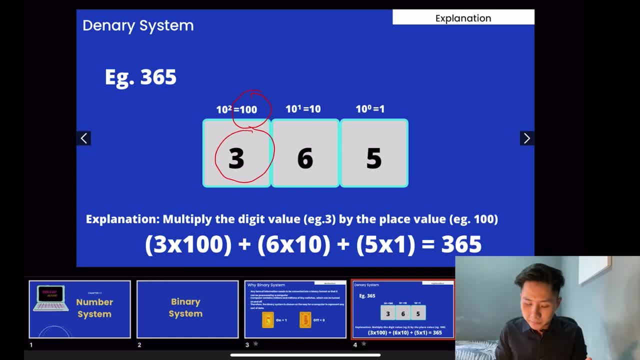 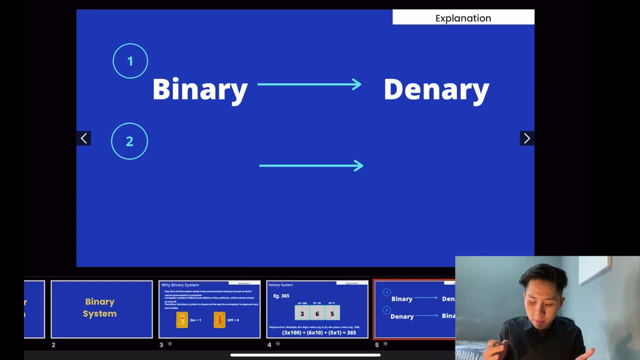 The only language that they can speak in is binary And therefore, in this video, we are going to learn how to convert binary to binary and binary to binary So that we can input numbers into the computer, So that we can transmit data to the computer using the language that they can understand. 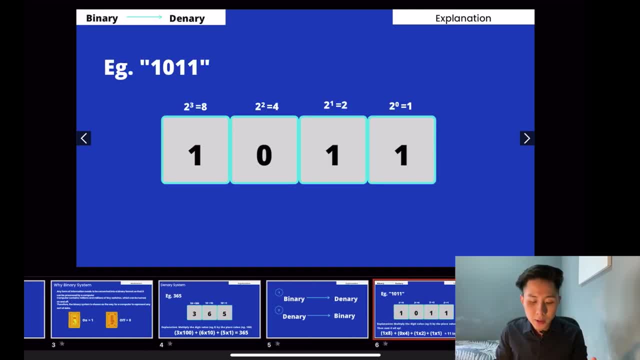 So let us start with the conversion of binary to binary 1011.. So how do we convert this binary value into a binary value that we can understand? And It is very similar to how we Understand binary system, Like what I mentioned how we obtain the binary. 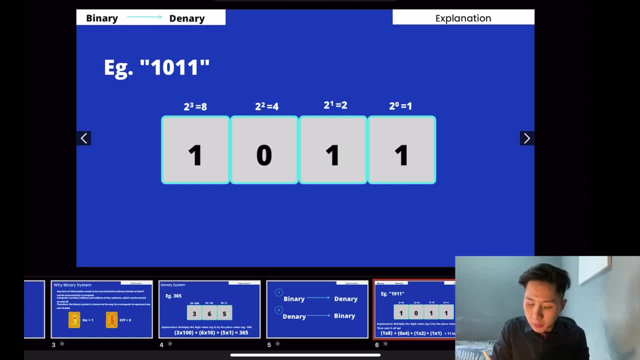 How we understand binary system is by multiplying the place value with the digit value, The digit value. The only difference here in binary system is that the place value of each position in binary system is different. Instead of The rightmost digit would have a value of 1.. 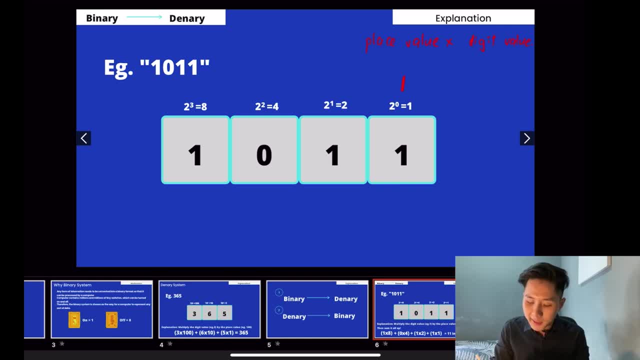 Which is similar to binary system, But the second rightmost: instead of the value 10, we have 2., Which is 2 power of 1.. Followed by 2 power of 2, which is 4.. And 2 power of 3, which is 8.. 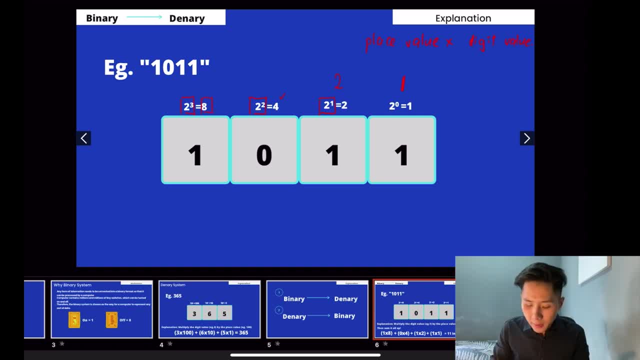 So on and so forth. We just increment the power, And to obtain the binary value of this binary, all we have to do is to multiply the place value with the digit value. So it would be 1 multiplied by 8.. Plus 0 multiplied by 4.. 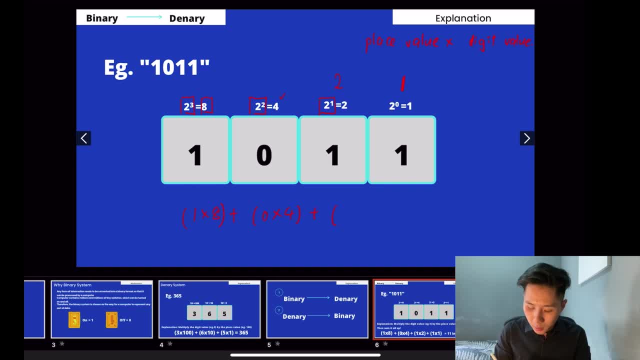 Alright, Plus 1 multiplied by 2.. Plus 1 multiplied by 1. And we would have the answer of 11.. So let us check if that's the correct answer. Yes, So we have the value of 11.. And the way we do this is just by multiplying the digit value with the place value. 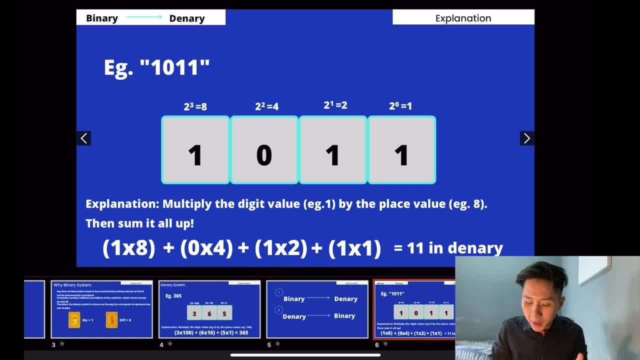 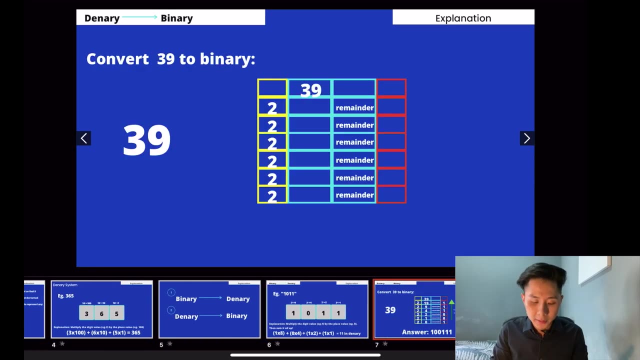 The things that you have to take note here is: what is the place value of the first position, the second position, the third position, and so on and so forth? Each value is multiplied by 2 in order to reach the next value. And to do it the other way around: how do we convert a binary value, the value that we all understand, into binary? 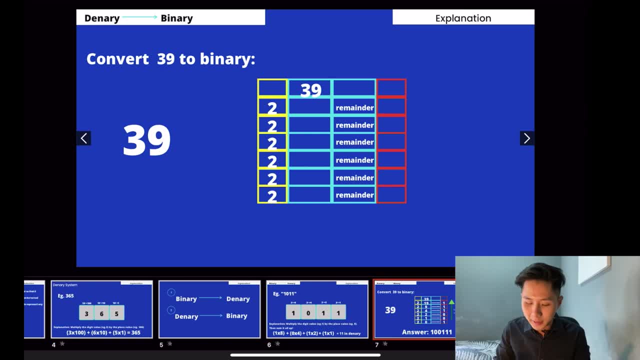 A language that computer can understand. So we have the value 39 here And the way that we can get the binary value of this. the binary value is that we will keep dividing it by 2.. Keep dividing it by 2.. 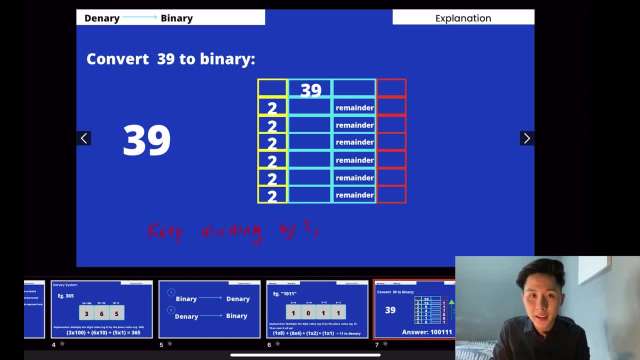 And use the remainder of the division to get our answer. So, for instance, 39, when we divide by 2, we got 19 as the quotient and 1 as the remainder. And if we were to continue to do this, 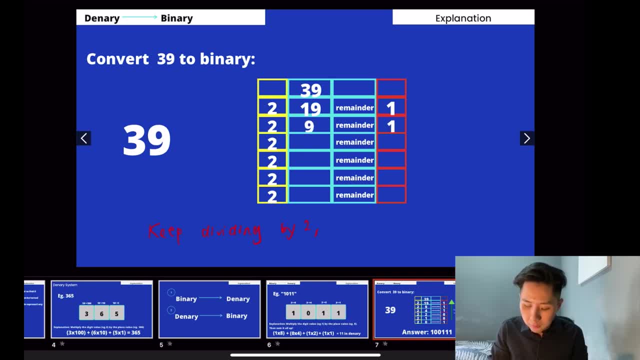 divide by 2, we got 9 remainder of 1,, 4 remainder of 1,, 2 remainder of 0,, 1 remainder of 0.. And, last but not least, 1 divided by 2, we got 0 as the quotient and 1 as the remainder. 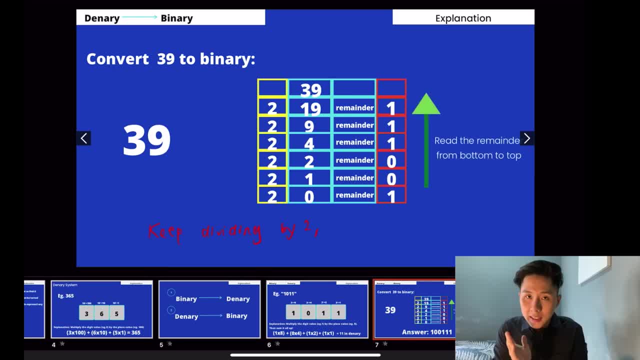 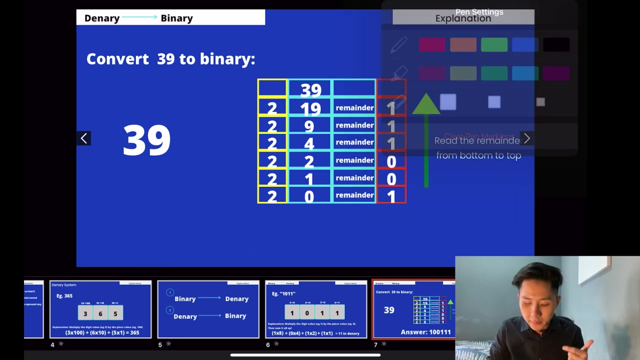 To obtain the answer, all we have to do is to read the remainder column from bottom to up, And by reading it from bottom to up we can construct our answer: 100111.. And this value here will be the binary value of the number 39.. 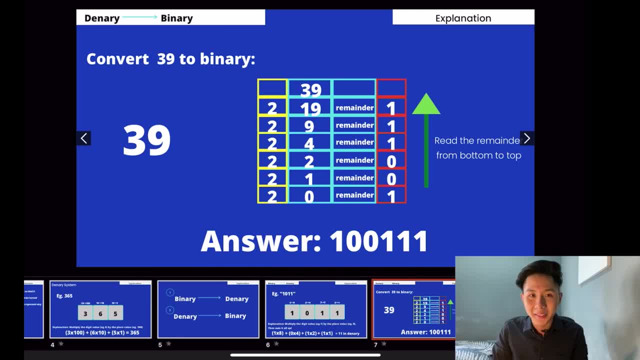 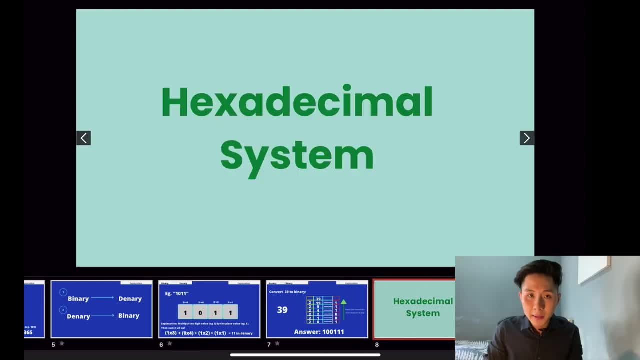 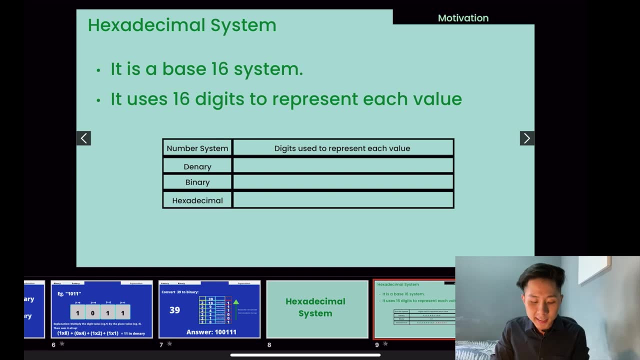 So let's check the answer: Yes, 100111.. And that's how you convert binary to binary and vice versa. Next up, the other number system that we computer scientists will care about is called the hexadecimal system, And it is a base-16 system. 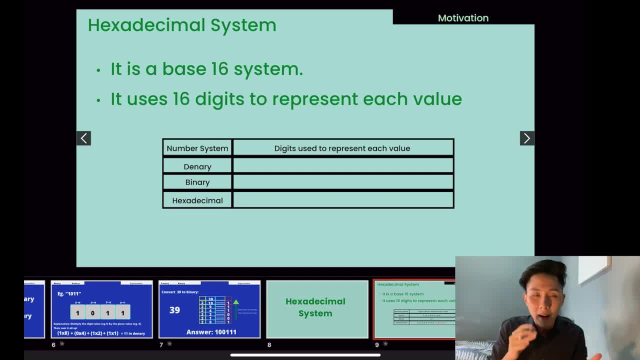 In binary, we know that there are only two unique values: 0 and 1.. Therefore, it is a base-2 system And in binary we have the value from 0 to 9, as you can see in this table. 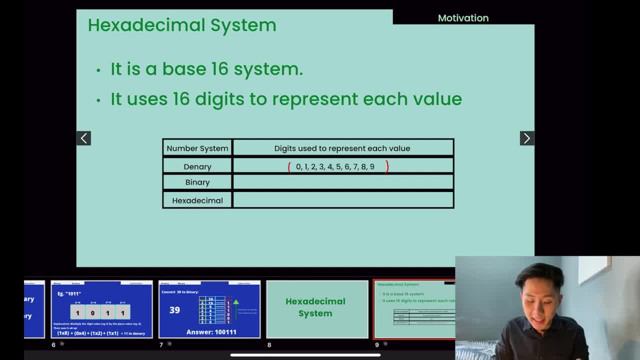 in which it is a base-10 system, because it has 10 unique values, Binary only 0 and 1.. And in hexadecimal there are 16 values, First up from 0 to 9.. And it's not followed by 10, but instead it's followed by a character, which is a to f. 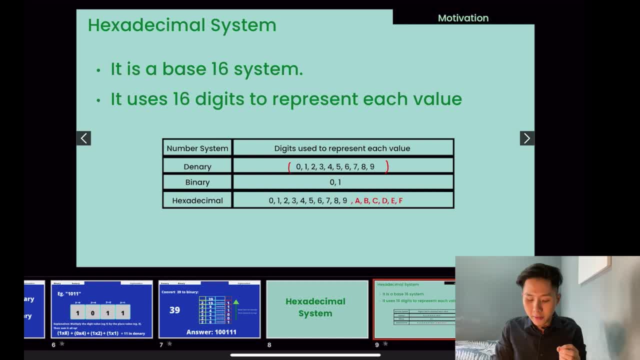 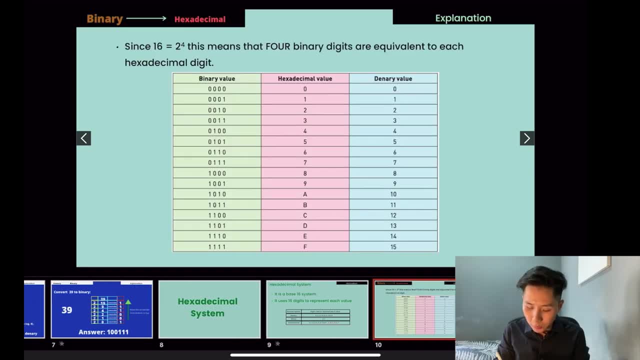 So in hexadecimal the unique values are ranging from 0 to the character f, in which a is equal to. We have a table here which maps binaries into hexadecimal and denary. As you can see, a in hexadecimal is 10 in denary. 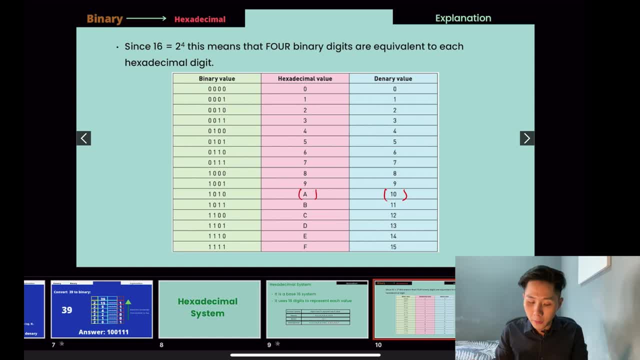 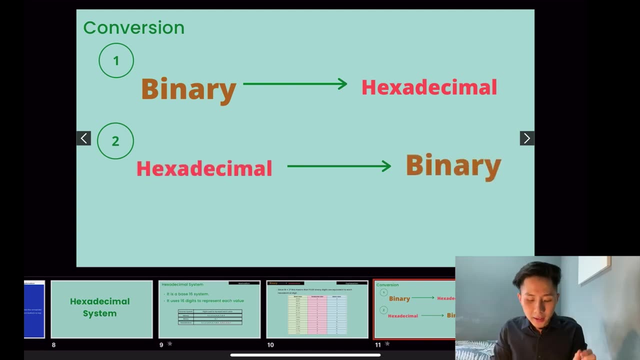 and b to 11, so on and so forth. This table is important. You might need to construct it during your exam to do the following question, which is the conversion of binary to hexadecimal and hexadecimal back into binary. So imagine this is the binary value that we have. 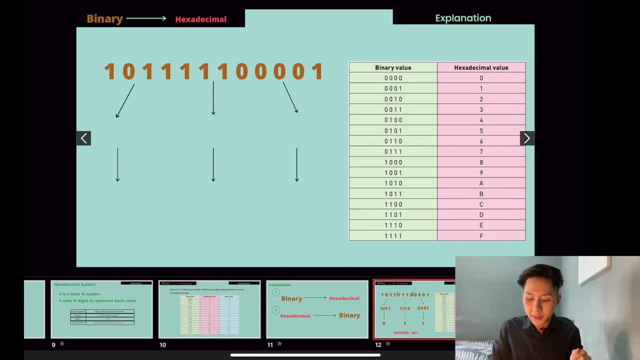 111000001.. And the way we can construct the hexadecimal of this binary. the first step is to split the binary into a chunk of four, So we have three chunks here- First chunk, second chunk and third chunk- And using the table that I introduced just now, 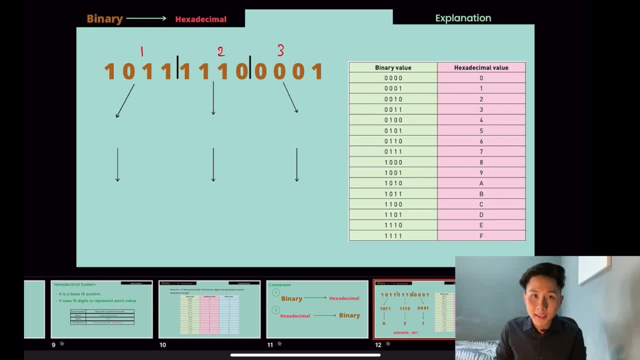 we can map this chunk of binaries into their respective hexadecimal value. So let's find 00001.. If we look at the table, it is 1 in hexadecimal. It's 1 in hexadecimal, so I just put 1 here And 1110, we have the value of e. 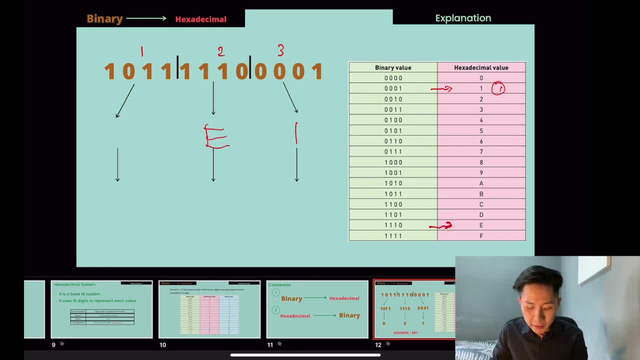 So we put the value e here- Sorry for the bad handwriting- And, last but not least, 1011, we have the value of b, So the full answer of this binary is be1.. So that's how we got our final answer. 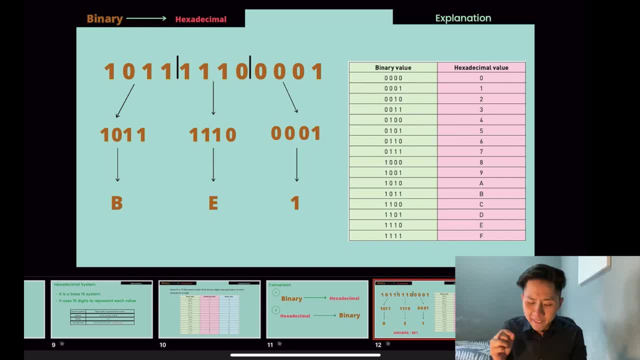 Easy right. That's why one catch for you is that in the exam you will have to construct this table by yourself. It won't be given, So it's important for us to construct this table by ourselves. So let's look into the other question. 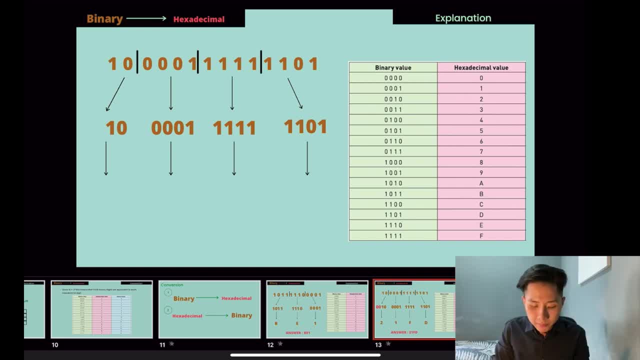 in which it's the same type of question, but here we have 14 digits in binary instead of 12. So that when we split this binary into chunks, we got four chunks, However the leftmost chunk, as you can see. 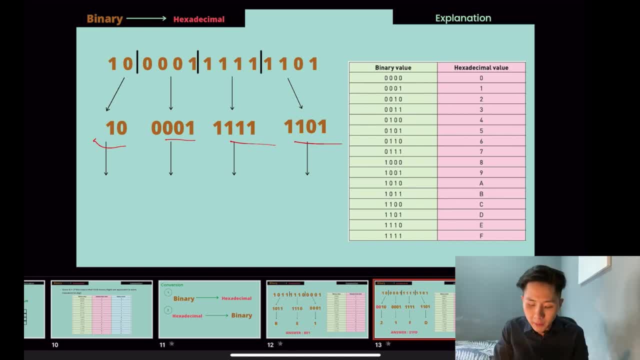 only has two digits, But we cannot find one zero in our table here. So what do we do? So, in this scenario, what you have to do is that you can just add the leading zeros to the value, so that you can refer this value back to the table. 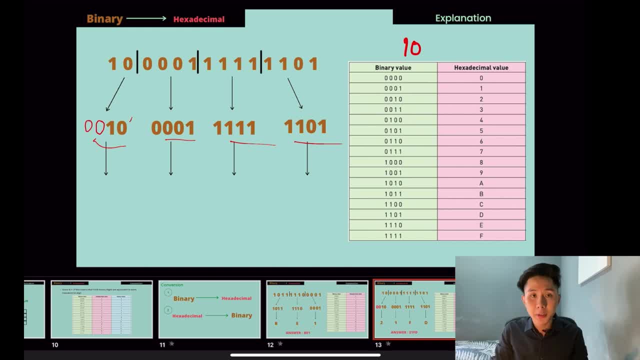 So by mapping these binaries into the table, we get the value of 2, 2, 1, f d. Feel free to check out the table to see if there's any mistake, right? So the final answer of it is 2, 1, f d in hexadecimal. 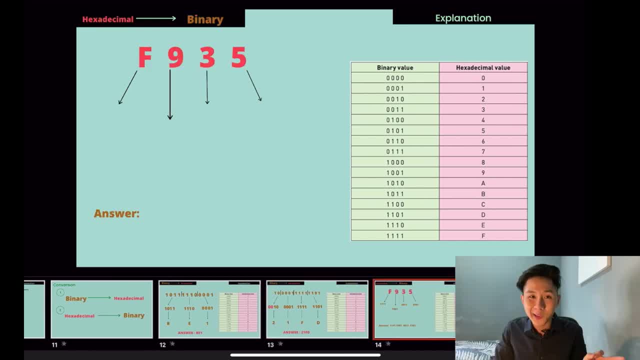 So let us do another question. This time it's the other way around, in which we convert the value, the hexadecimal value, back to binary. So I guess you might have already know how to do this. Again, we map those values back into. 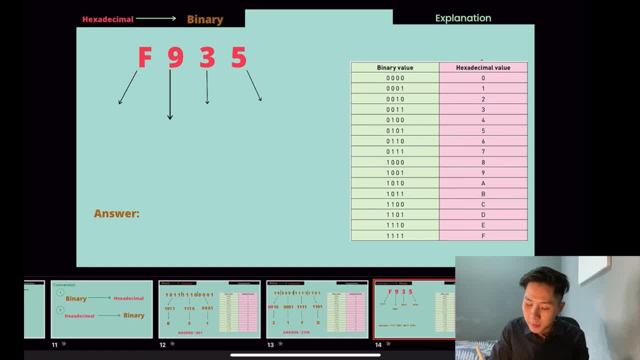 their respective binary value, which means we are referring from the right column to the left column. So the value f: we have four 1s. The value 9, we have 1, 0, 0, 1, as you can see here. 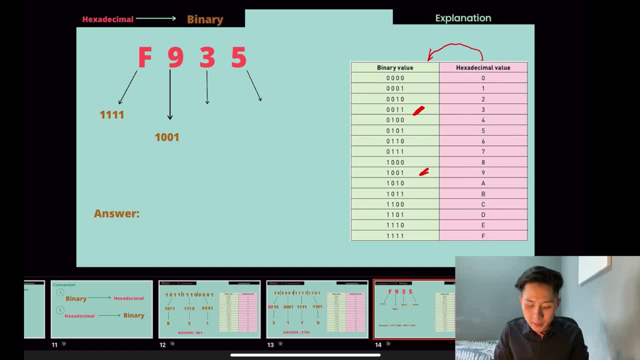 3, we have the value 0,, 0,, 1,, 1.. And 5, we have the value 0,, 1,, 0,, 1.. And all you have to do is just concatenate all these strings together to form our final answer. 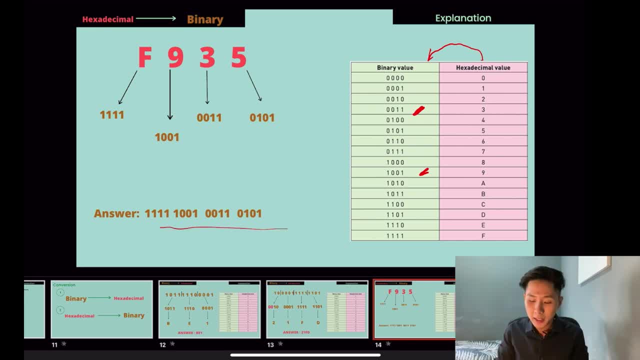 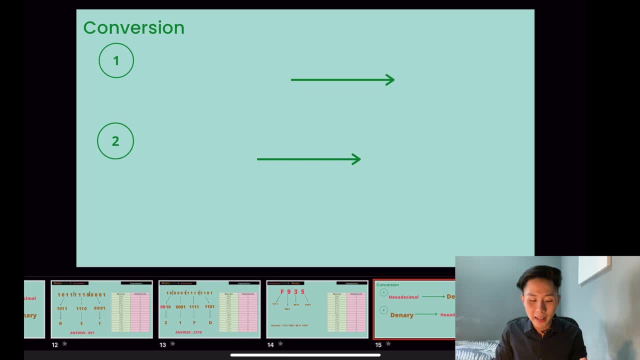 So that's how you can convert hexadecimal to binary. In my opinion, they are the easiest question that you can see in the exam. all right, So next up, the last two conversions that we need to do in this subject is to convert hexadecimal instead of to binary. 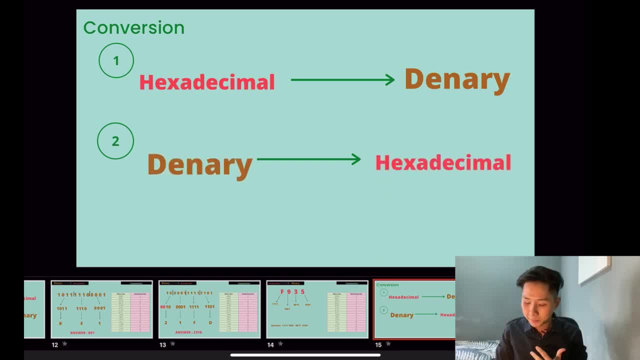 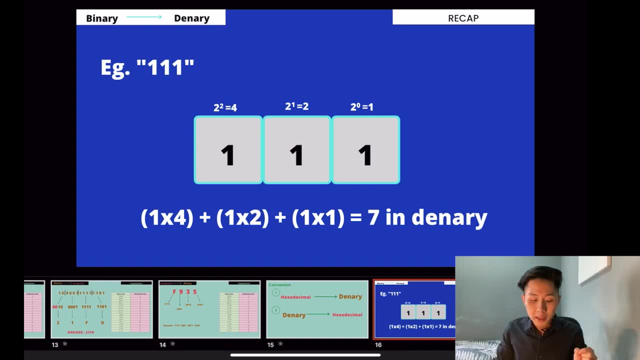 We are going to convert it into denary and vice versa. So the method to do this is very similar to how we convert binary to denary. If you remember, the way we convert binary to denary is that we multiply the digits. We multiply the digit value to the digit value. here. 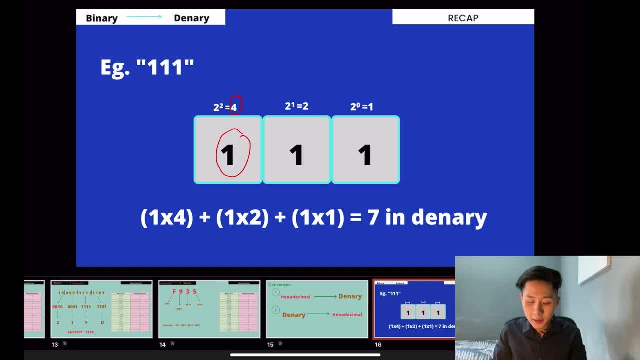 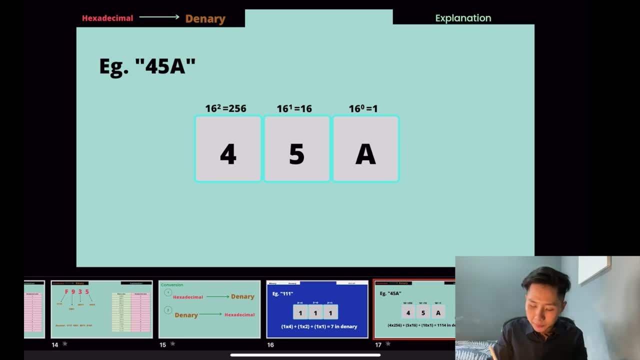 to the place value here. all right. So in hexadecimal the only difference is the place value. So the rightmost place value is still 1.. But the next value, instead of 10,, instead of 2,, it is now 16.. 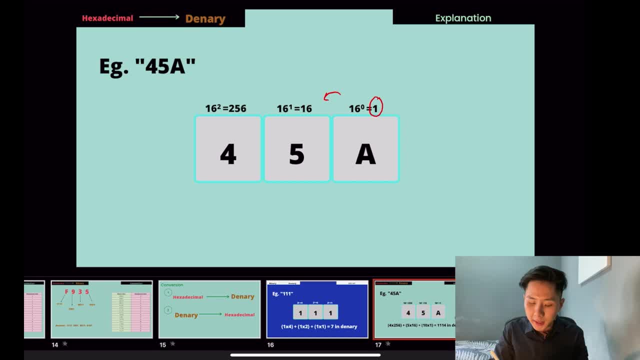 Remember, hexadecimal is a base 16 value. So we got 16 power of 1, we got 16. And followed by 256.. It's gotten it from when we multiply 16, two times 16, to the power of 2.. 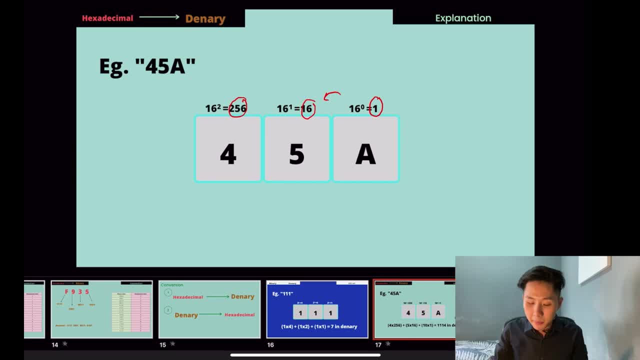 And again, now we can do the basic thing, But before that we have to remember that in hexadecimal there are some characters. So before we do our conversion, we do need to convert this character into value, For instance A. we need to convert it into the value 10.. 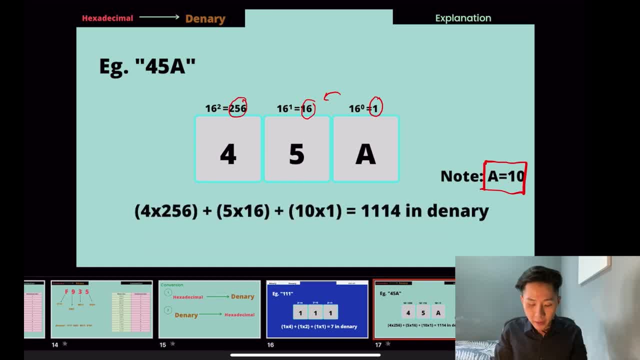 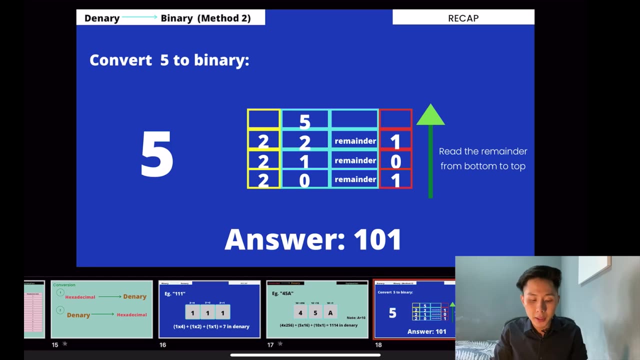 So we can just do the basic stuff By multiplying the place value with the digits value And we have gotten our answer here. OK, Feel free to try it yourself. So next up, we're going to convert denarii into hexadecimal. 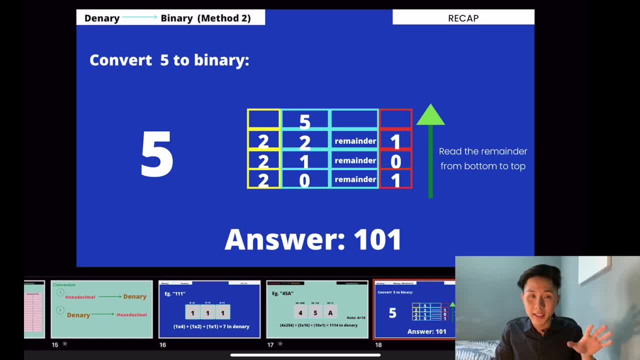 And the way we do this is very similar to how we convert denarii to binary. If you remember, the way we convert the value 5 to binary is that we keep dividing it by 2. We have the remainder. We read the remainder from binary. 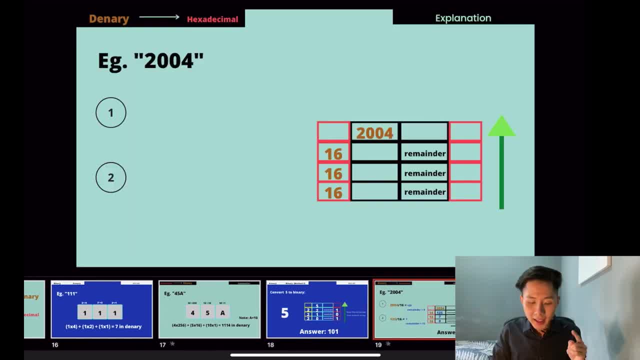 And bottom up. OK, So we have an example here. How do we convert the value 2004 into hexadecimal value? So instead of dividing the value by 2, which occurs in binary- we will divide it by 16.. And if we were to do this, 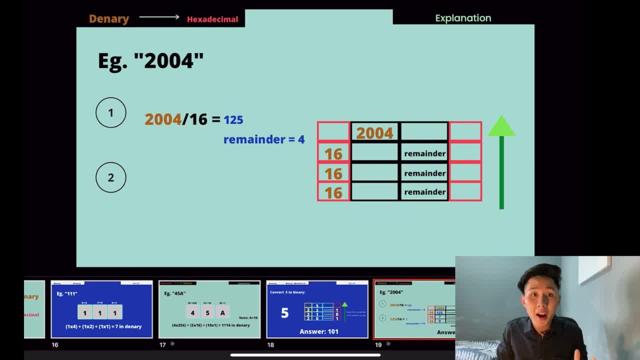 2004,. when we divide by 16, we got a value of 125 as our quotient and 4 as our remainder. So we just write the value back into our tables here And let's continue to divide this 125 by 16.. 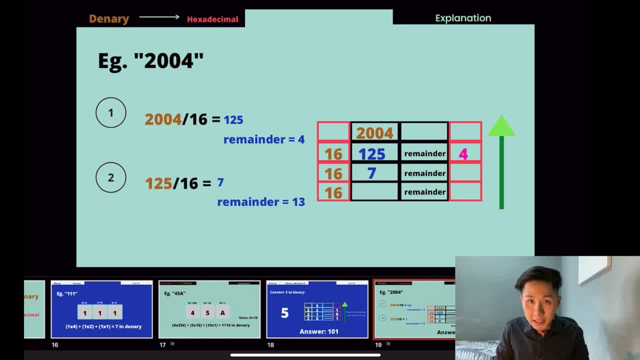 We'll get the value of 7, remainder of 13.. But remember, in hexadecimal there is no value 13.. 13 is represented by the character d, alright, And so on and so forth. We just divide 7 by 16.. 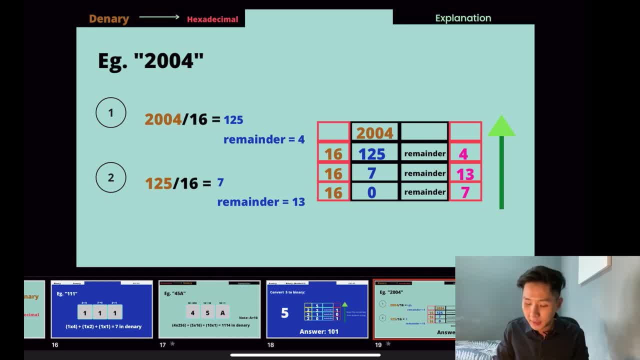 We got 0 as quotient and 7 as our remainder. To construct it, we read the remainder from bottom up And we'll have the value of 7d4.. So 13 is equivalent to the value d in hexadecimal, And that's it. 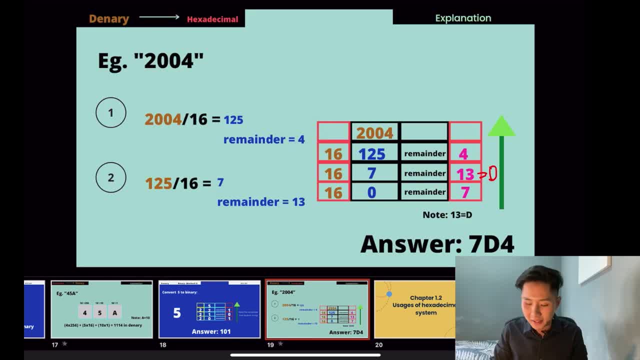 That's all the conversion problems that we need to do. alright, Feel free to re-watch certain part or comment. if you have any doubts on how to do this question. I will try my best to answer And next up, having learned about the hexadecimal system. 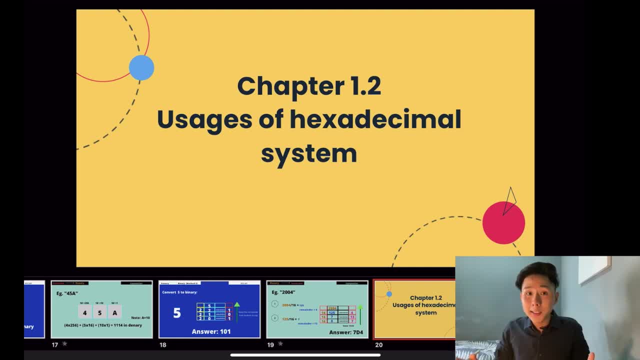 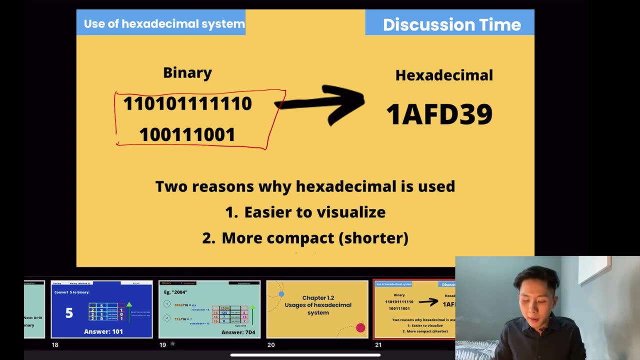 we are going to have a look on what are some of the usages in computer science. Why do we need them if we already have the binary system? And just look at this diagram. The binary value here is corresponding hexadecimal value. is this? I won't do the conversion part. 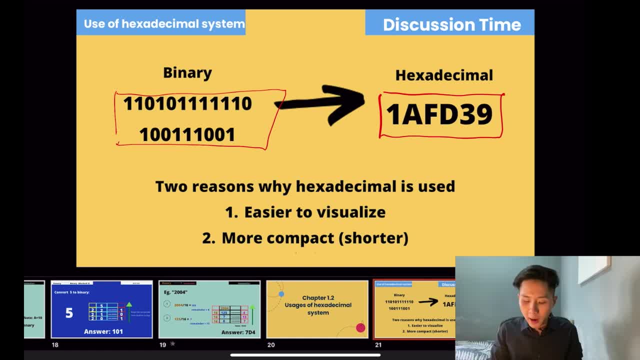 You guys can try it yourself. And there are two reasons why they are used. The first one is, as you can see, hexadecimal is easier for us to visualize. There are a lot of one and zero here in binary. It would be difficult for programmers. 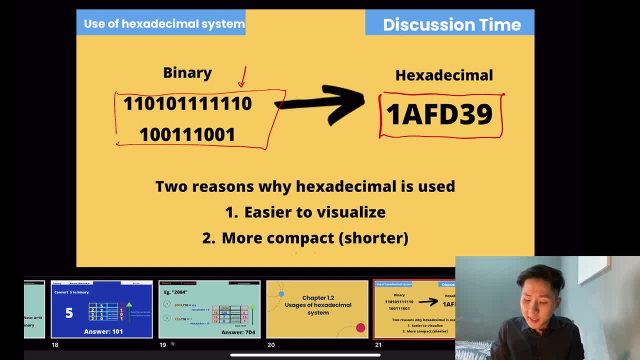 or computer scientists to read data in this way. Instead, it's easier for us to look at the hexadecimal value, which leads us to the second advantage of hexadecimal, which is it is more compact and shorter. Remember, four binary digits is equal to one hexadecimal value. 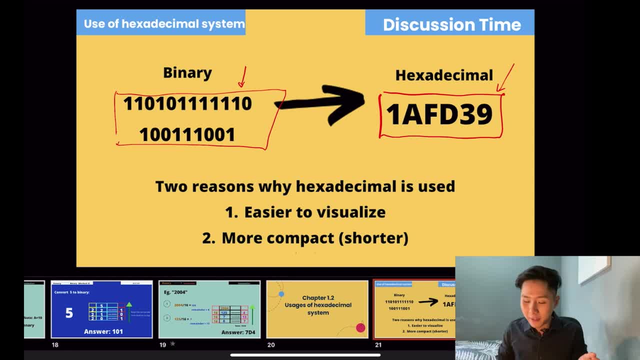 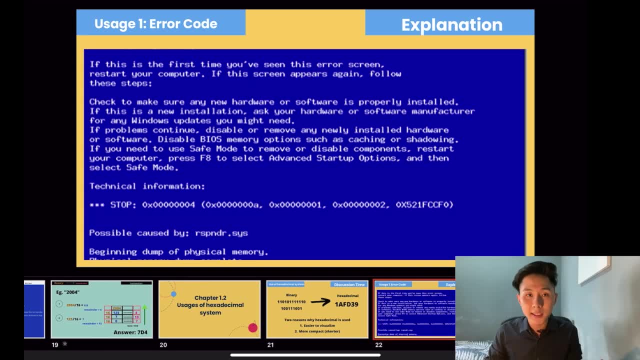 So that reduces the length of the data by four times when we use hexadecimal. So there are four usages of hexadecimal system. The first one is arrow codes, in which it tells the programmers where the arrow is located by putting up all this hexadecimal value. 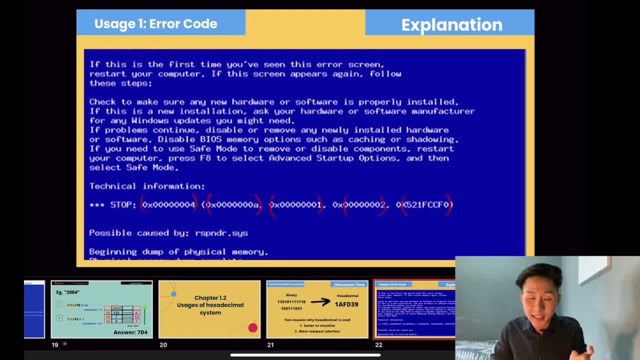 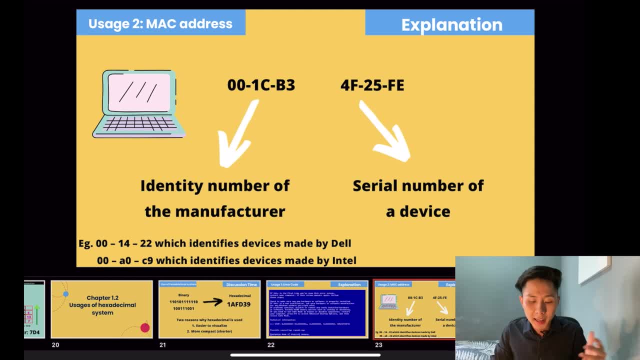 If you can see here, these are all hexadecimal value. So that's the first usage of hexadecimal And the second usage of hexadecimal system is the MAC address. MAC address is basically an identifier for your device, like laptop and smartphones. We'll go into that more in details. 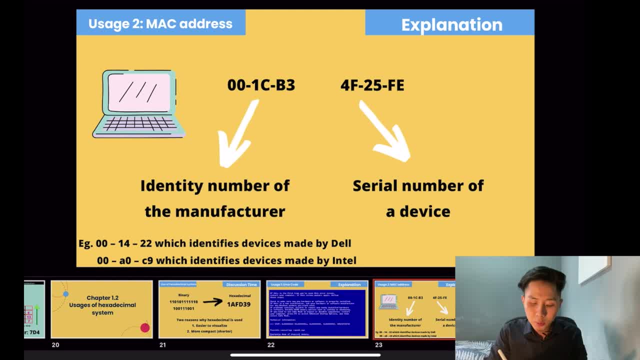 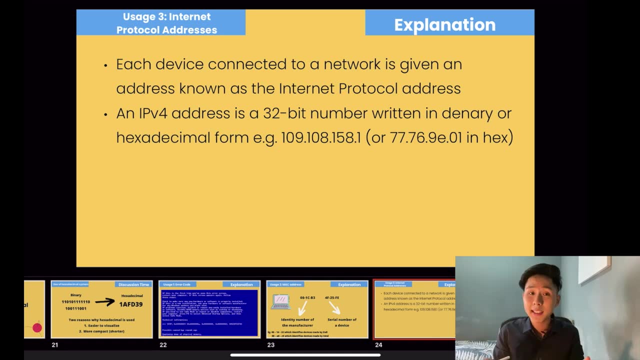 in chapter three. So as you can see the MAC address of a device, feel free to check your own MAC address in your computer. they are also represented in hexadecimal And the third usage of hexadecimal is the IP address, which is an address given to a device. 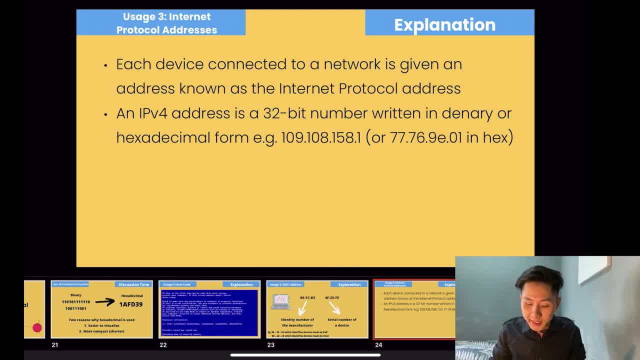 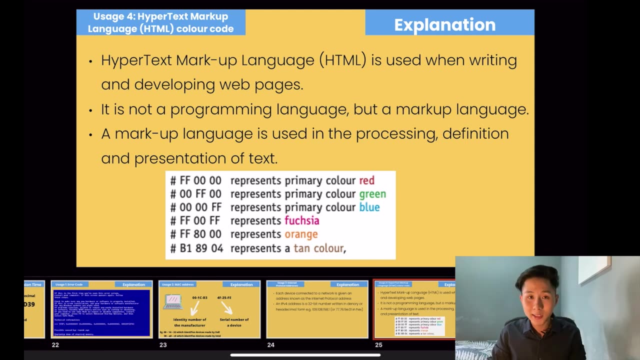 when it is connected to a network, So for instance an IP address. it could be represented like that- see the red bracket- in hexadecimal instead of in binary. So the last usage of hexadecimal system is called the HTML color code. HTML is basically a language. 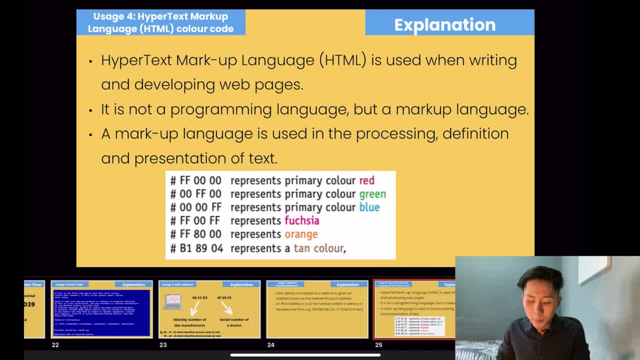 that programmers use to develop websites. It's not a programming language but a markup language. So when you're making a website, there are certain colors that you might want, and you would encode this into your in hexadecimal, All right. So to summarize, 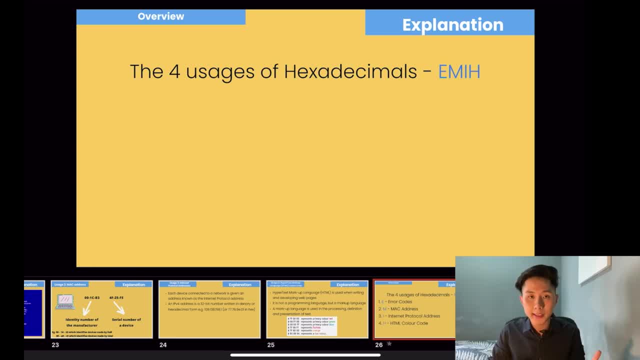 so, because this is a very commonly asked exam question in IGCSE. therefore, I use a mnemonic to help me memorize the four usages of hexadecimal system called the IMME. So E stands for arrow codes, M stands for MAC address, I stands for IP address. 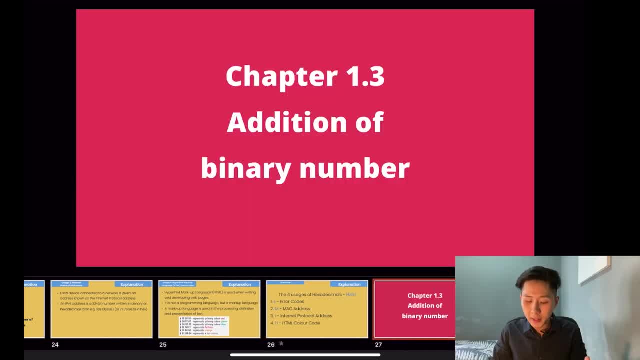 last but not least, HTML color code. All right, Having talked about hexadecimal system, let's move on to the addition of binaries value. How does computer carry out addition, For instance in our calculator apps? how do they multiply values and add values? 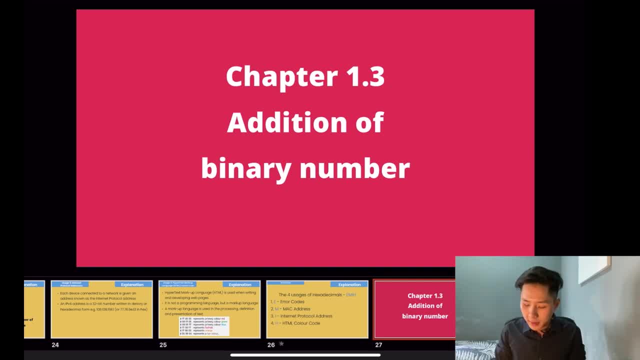 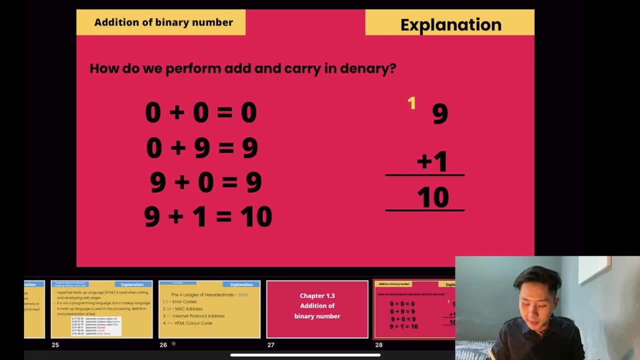 So this is what we're going to look into the next two segments. So if you remember how we carried out addition in binary, is that using this old school method here? All right, Let me change another color for this background. So this is how we perform addition. 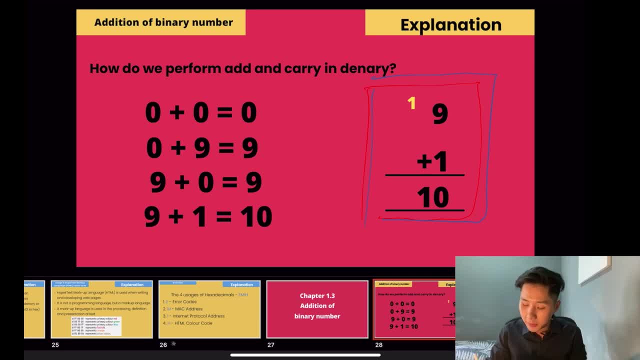 in binary system. So nine plus one, we have the value 10.. So 10 is our value, residual value, and one is our carried over. So we have. But in binary it's a little bit different, If you remember. 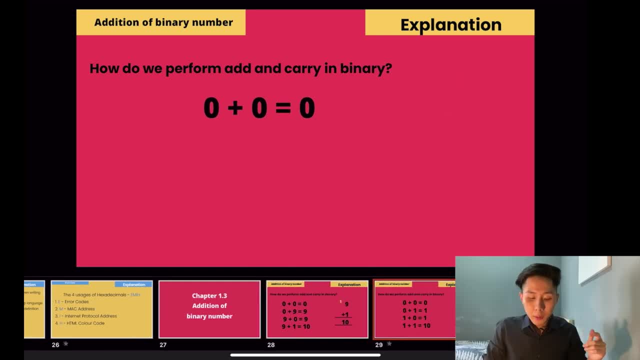 binary only have two unique values. So if we were to add zero and zero, obviously we're going to get zero. Zero plus one, we're going to get one. One plus zero, we're going to get one again. But if we were to do 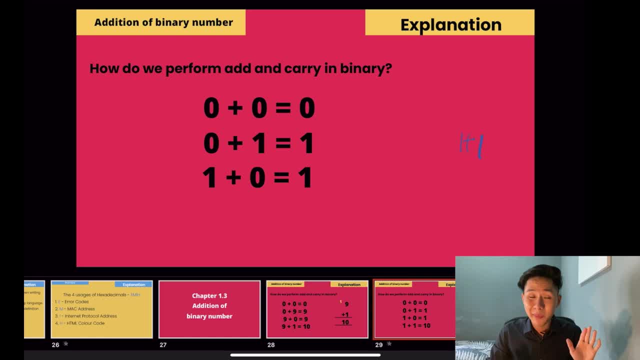 one plus one. remember, in binary there's no value called two. What it will do is that one plus one is equal to one zero. One plus one is equal to one zero, And how it works is that when we use one plus one. 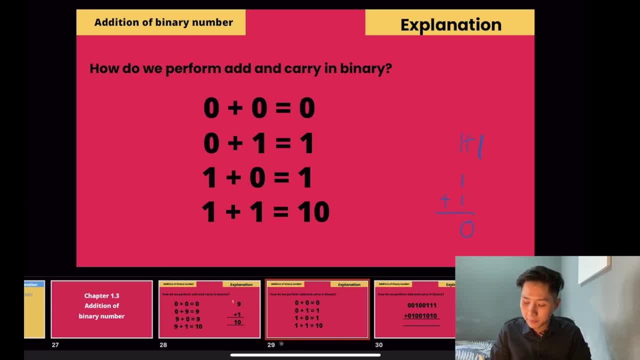 we'll get zero with a carried of one, because one is the maximum value in binary And we just bring this carry down. That's how we get the value of one zero. If I were to add one plus one plus one, I will get the value of one one. 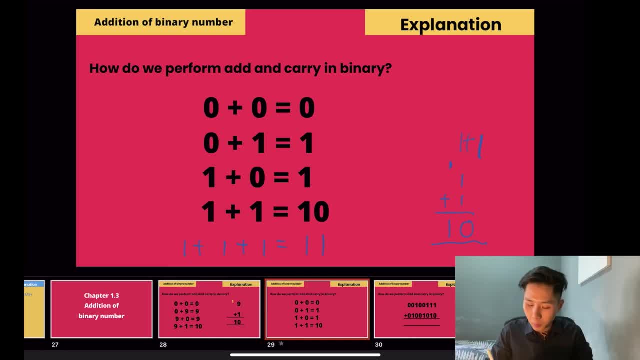 It's not eleven, It's called one, one which is one plus one plus one. If I were to do it here, we get one with the carry of one. So that's how we add binary values. And let's try out an example here. 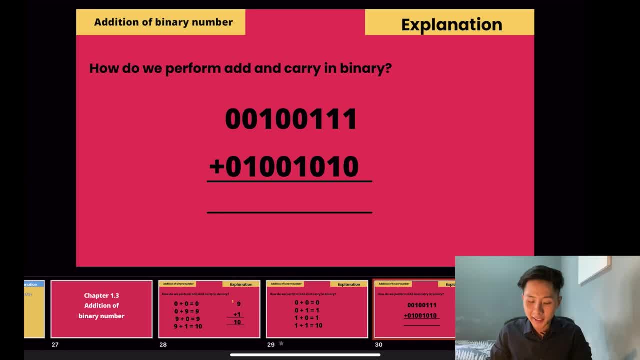 How do we perform at in this example? So you can just go through with me: One plus zero, we got the value one. One plus one, we got the value of one zero. So our value here is zero with a carry of one. 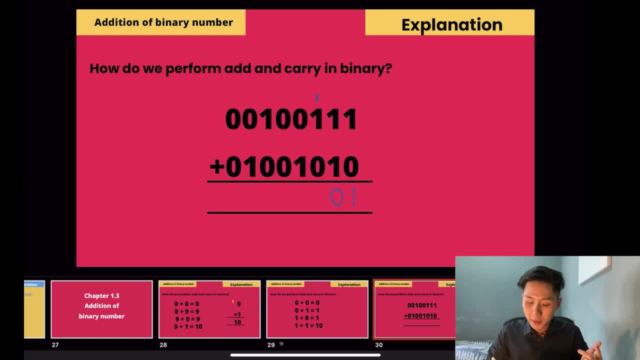 And move on. We have one plus one and we'll get one zero again. So again, zero with a carry of one. One plus one. zero with a carry of one. One plus zero. plus zero, we get a value of one with no carry. 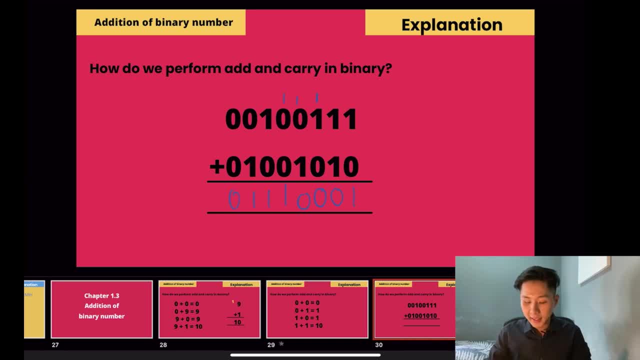 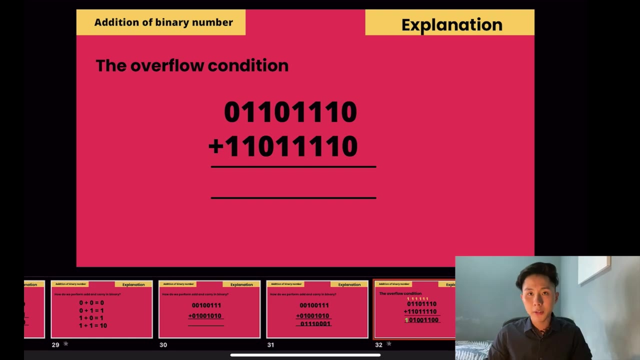 One plus zero, one, Zero plus one one. So that's all. That's how we convert this value into, That's how we add two binary numbers together. So that's the answer. And here I want to introduce another condition called the overflow condition. 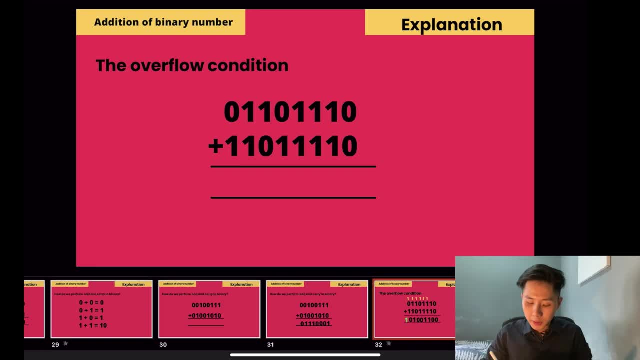 It might happen. So let's do this addition again. You can pause the video to try it yourself. Zero plus zero. we got zero, One plus one, one. zero, One plus one plus one. one with a carry of one. Again one with a carry of one. 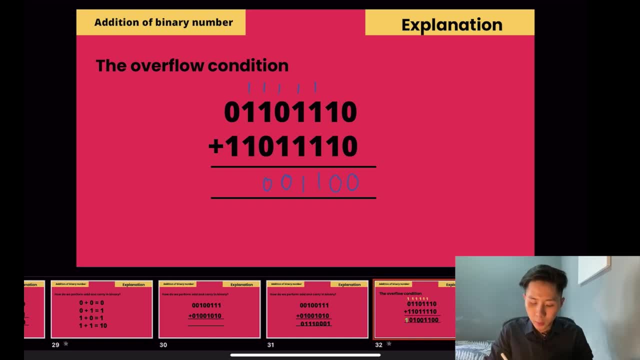 Zero, one. zero Carry of one. One plus one. one Carry of one. One plus one. zero See, We have generated one plus the ninth value. One plus nothing, We get the value of one. So when we add these two binary numbers together, 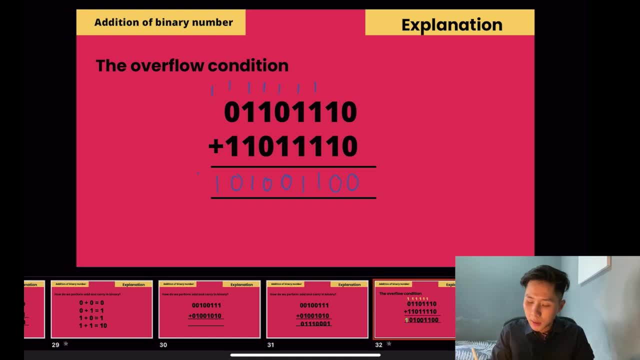 we have generated an extra, an extra digit here, An extra one value here. Okay, what is the big deal of this? right? This is: we care about this thing because when we are learning about hardwares, we know that certain 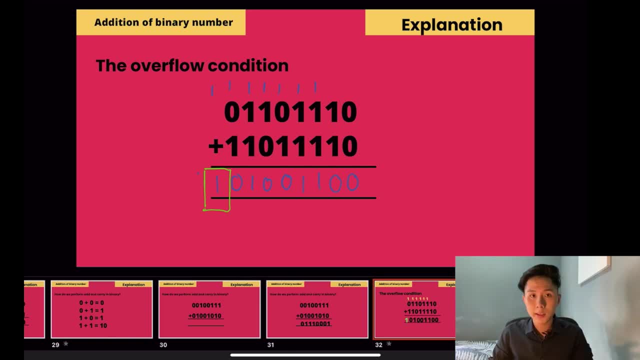 that the component that stores this value is called a register, And sometimes register might have a fixed size. What if the register that store this value only can store eight binary bits? If this happens, the extra bits that are generated here will be: oh, let me adjust this. 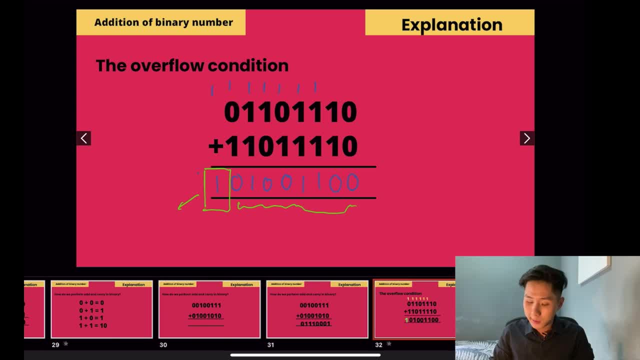 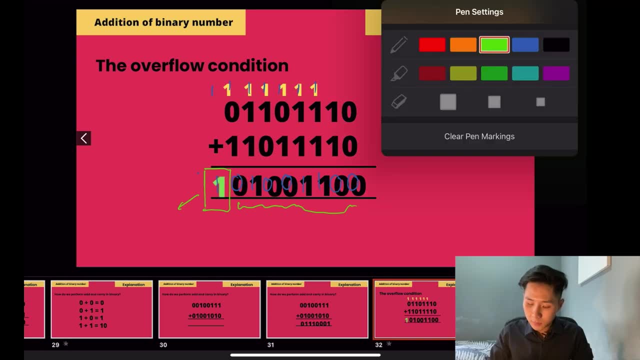 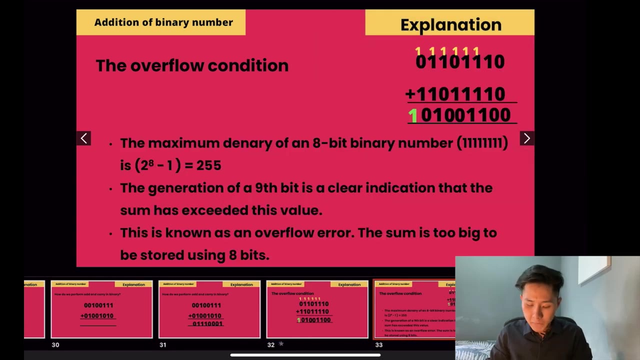 The extra bit that's generated here will be lost. Alright, if I were to do this all again. So this is the value that we'll get. So let me clear my drawing, Alright, See, So the overflow condition is when a ninth bit is generated. 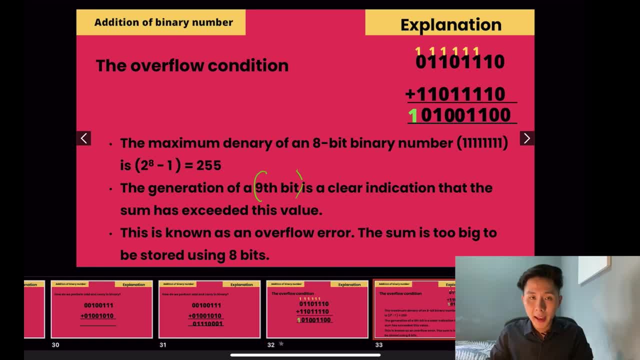 This means that the value, the summation, the value, the result of this summation, has exceeded the value that eight bit binary numbers can store. And eight bit binary numbers here we have eight ones here. If you check, the value of this is 255.. 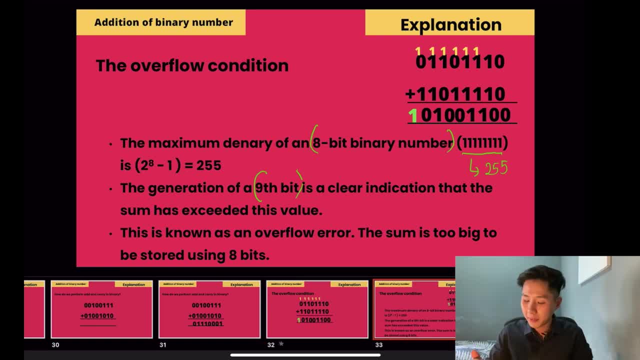 But we know that when we add two numbers together, there is a chance for the result of this summation to exceed this value, And this is how the ninth bit is generated. This is called an overflow error, Which means there is a risk that 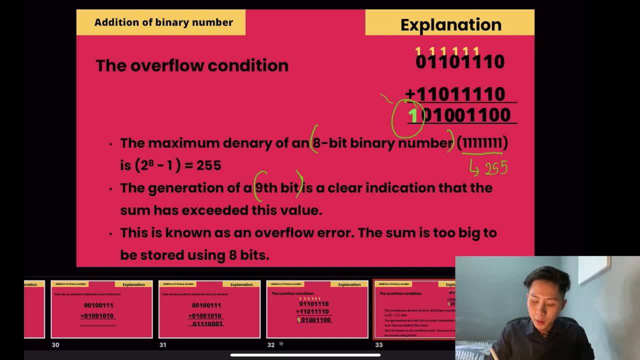 this extra bit generated here, the green color one, will be lost. The sum is too big to be stored using just eight bits. Okay, So that's how we do addition and the overflow problems that we might face when we do this. 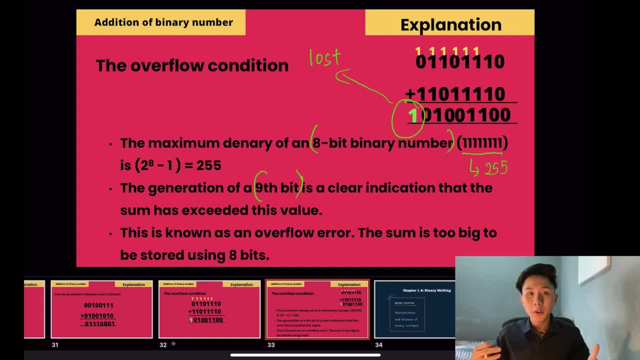 In the IJCIC exam. they might ask, they might give you just two binary numbers and ask, if okay, does overflow problem occur? You have to answer this yes and give the reason of it Why? Because the ninth bit. 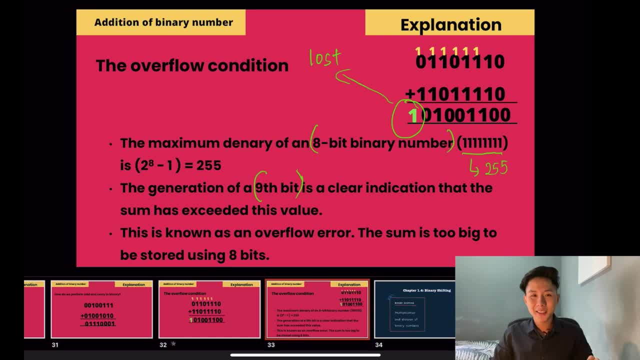 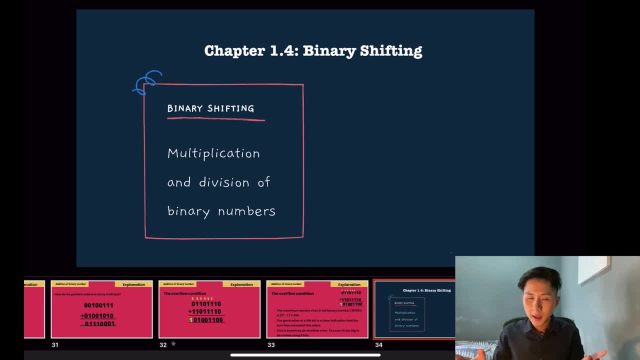 has been generated. So, having learned about how to add binary numbers, now we'll move on to how do we multiply and divide binary numbers. Think about it, It's necessary. There is a plus and divide functionality in your computer, right? 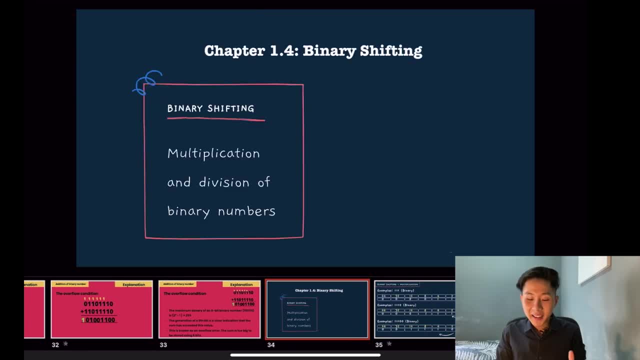 So let's learn how do we do this. The method that we use to multiply and divide binary numbers is called binary shifting. Binary shifting: In essence, we are basically shifting the binary numbers. So let me give you an example here. 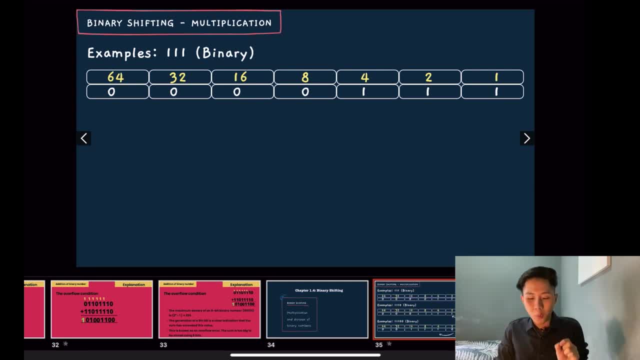 So we have the binary value, one one one here And one one one in binary. we can just multiply. use back the method that we learned: multiply the place value by the digits value, which we will get the value of seven here. 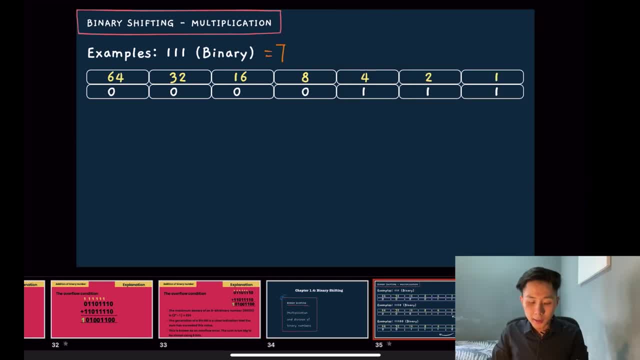 We'll get the value of seven. Okay, So let's try to shift this binary value one, one, one to the left, In which we will move each digit one, one place to the left. Alright, So when we move. 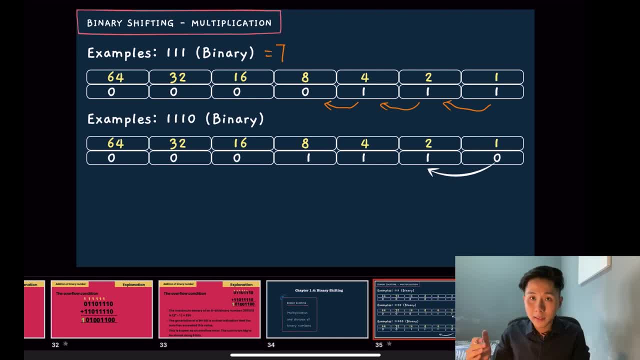 one, one one to the left. we got one one one zero instead, And I want you to observe this, the effect of this shifting So from the table, we know that the binary value is eight plus four plus two. 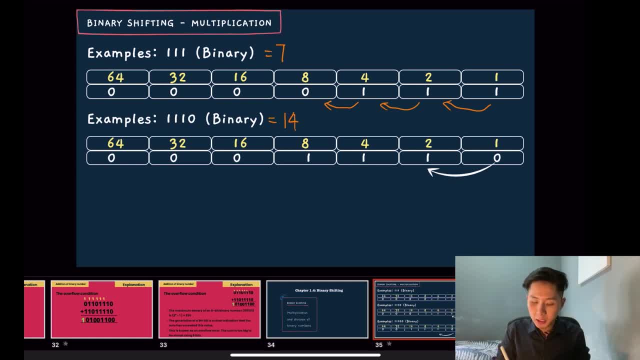 in which we get fourteen. Alright, Hopefully you are starting to observe some pattern here, So let me just move this binary. one more places to the left. So one more places to the left. we will have one, one, one. 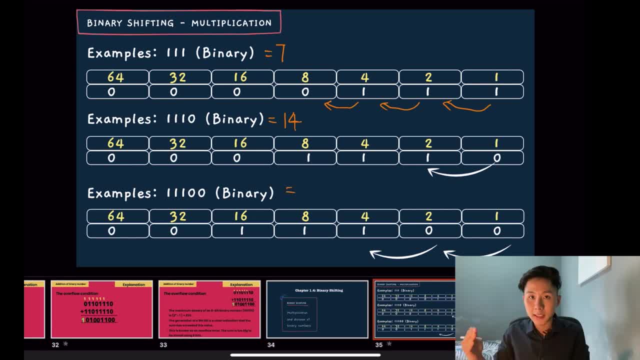 zero, zero. And in binary this value is sixteen plus eight plus four, in which we get the value of twenty-eight. Alright, So we have a pattern here When we shift the value of the binary to the left by one digit. 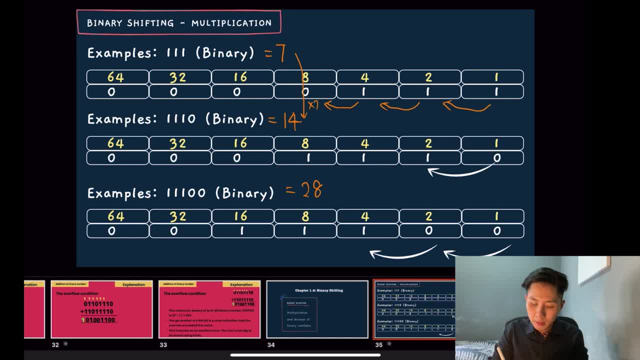 the value of it is actually multiplied by two, And if we were to shift it again, we will multiply it by two again. So that's the pattern of it. It's that when we shift the binary value one place to the left, 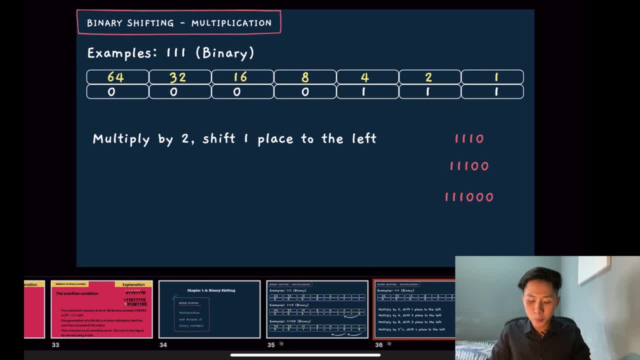 we are multiplying by two. If we were to shift it two places, we are multiplying by four. Three places, we are multiplying by eight. And by following this pattern, if we were to move n places to the right, we are multiplying the value. 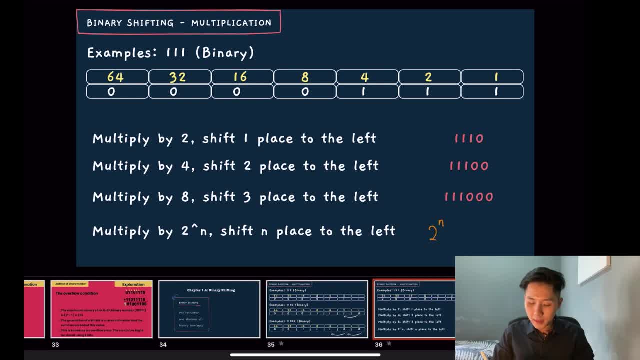 by two to the power of n. Okay, If you can see, here, when we move one place, we got the value two, which is two power of one. When we move two places, we got two to the power of two, which is four. When we move: 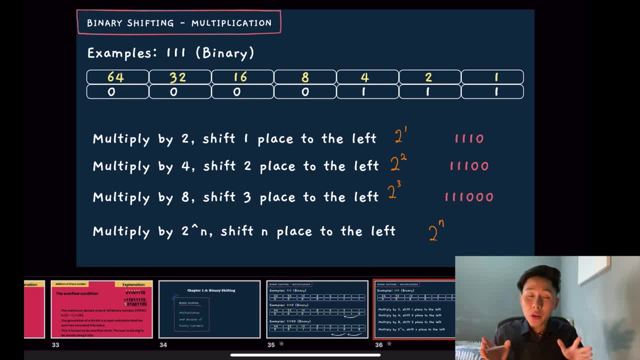 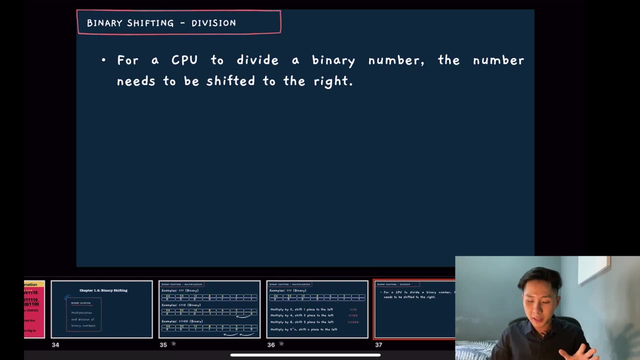 three places. we get three places to the power of two. So this is how we multiply a binary value with shift the binary value one place to the left, And to do division we can do the exact same thing, but we are, we just change. 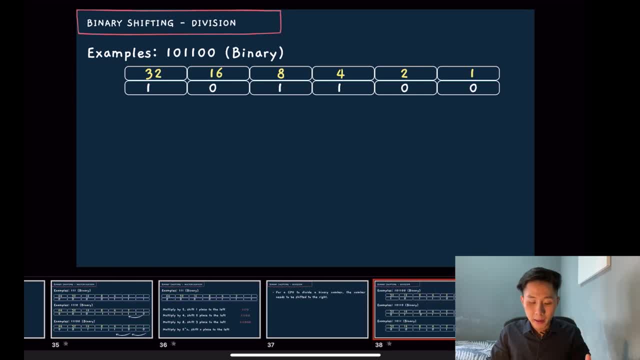 the direction of the shifting. So for a CPU to divide a binary number, the number needs to be shifted to the right. So two plus eight plus four will have the value of forty-four. So if I were to shift this value one places. 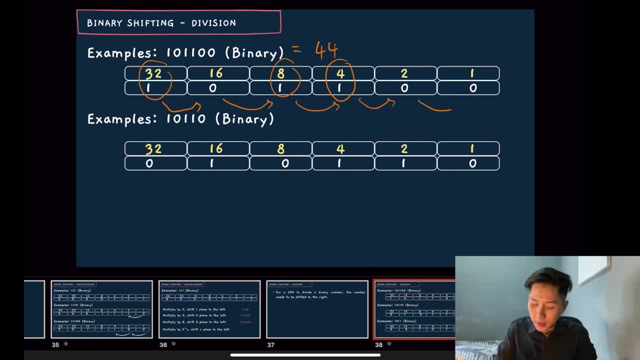 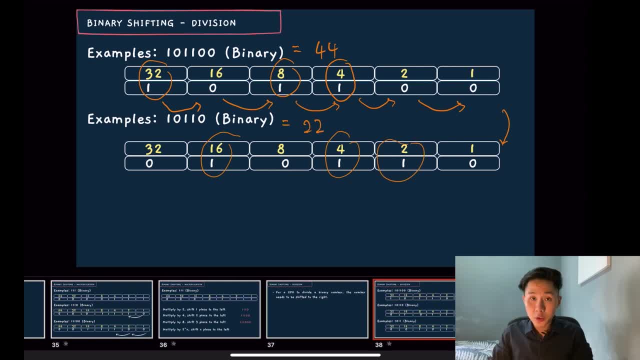 this value in binary it's eight plus two plus one, which will get eleven. So from the value here hopefully you can see the pattern. Forty-four to twenty-two is division of two. Twenty-two to eleven is again division of two. So 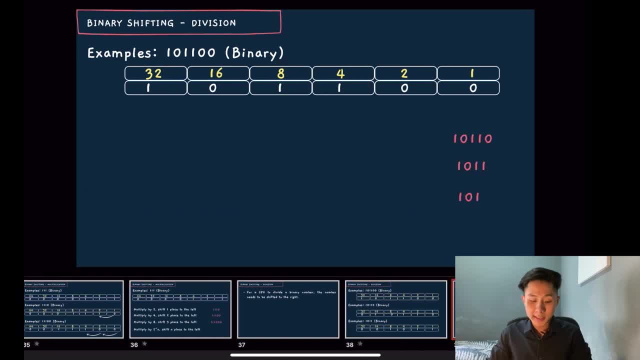 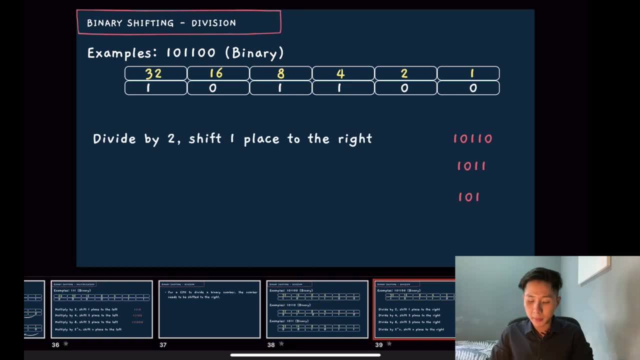 the same theory persists: One oh one, one oh oh. if I were to shift one place to the right, the shift one place to the right is division by two, Two, four, three places divided by eight in the formula. If I were to shift, 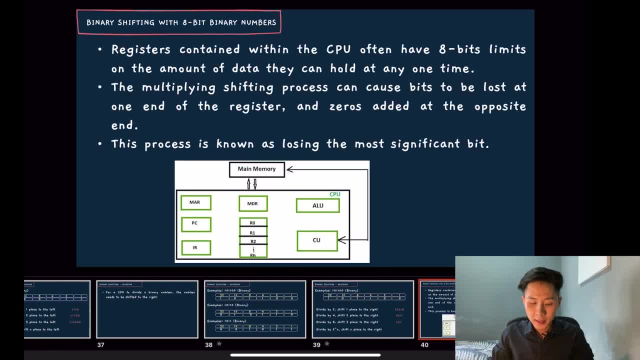 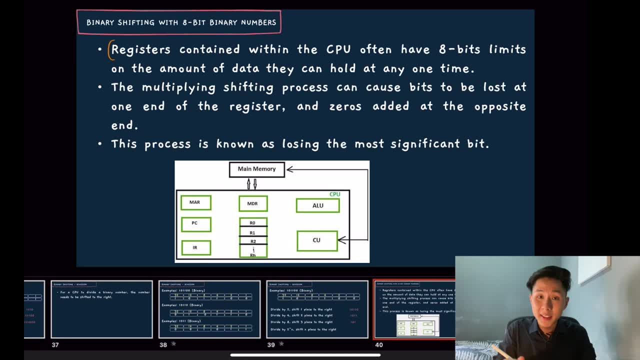 n places to the right. I'm actually dividing a value by two, two to the power of n, So okay. So here they say that register contains within the CPU. Register is a component that stores all the bits that a computer needs. We'll talk more. 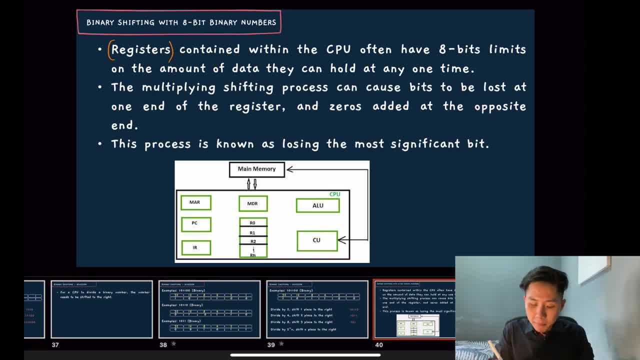 about it in chapter three- And the amount of data that it can hold at one time is limited because the number of bits that they can store is limited. Therefore, the multiplying shifting effect- multiplying shifting effect- can cause bits to be lost at one end. 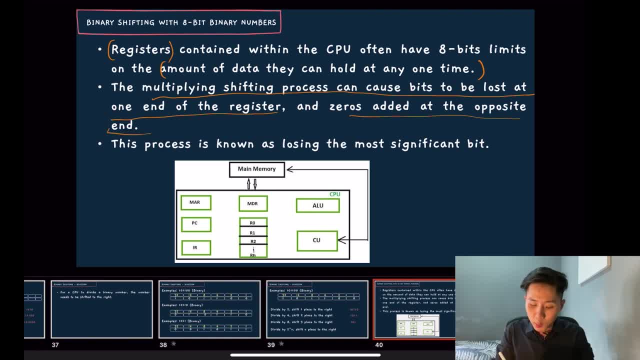 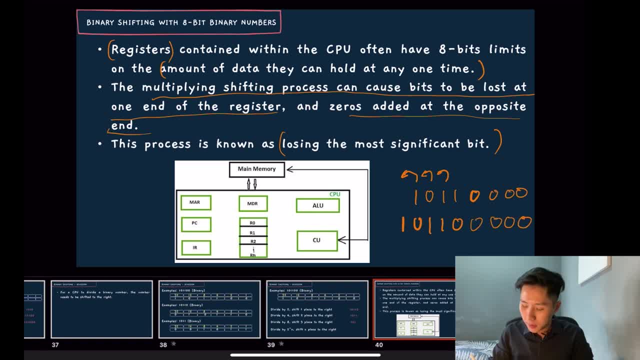 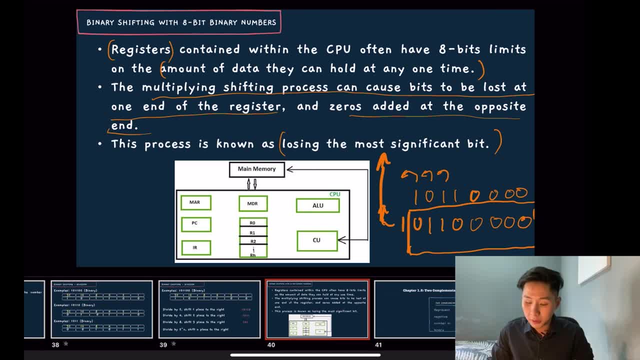 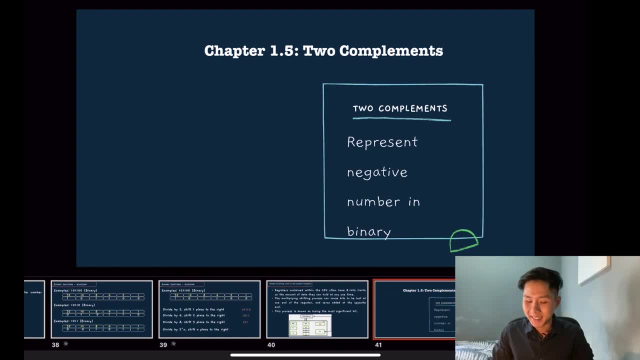 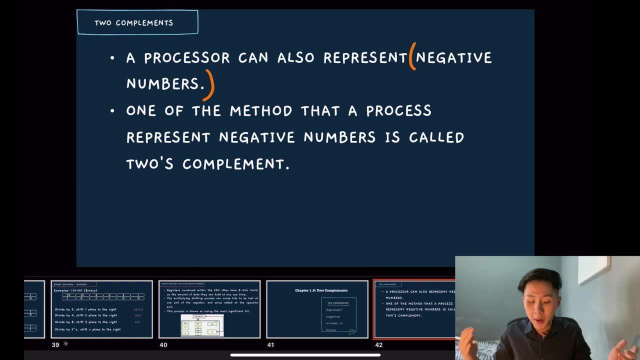 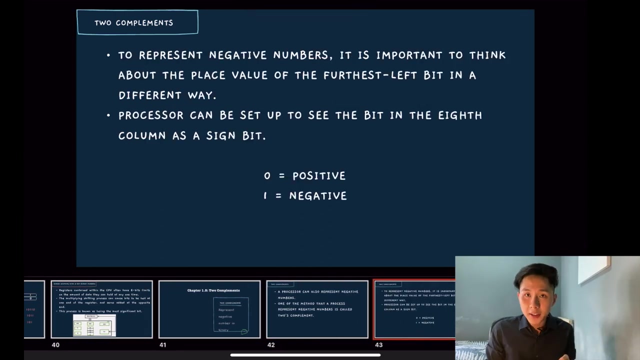 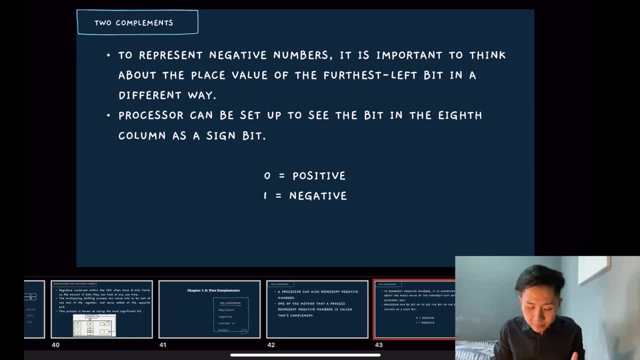 it's learning. the conversion we have to take note of this is that in two complement, if the starting digits starts with the value of zero, this means that it is a positive value, and if the leading this is one, this means that it is a negative value. for instance, let us have this value in two's complement. 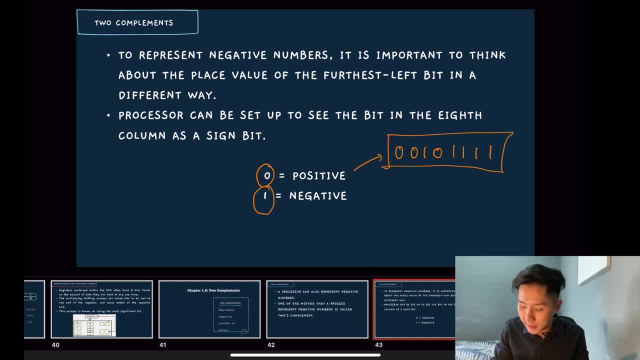 without having to calculate this, we know that this is a positive value because it's leading value is leading bit is zero. and, on the other hand, if I were to have a value like that without calculating it, we know that this is a negative value because it has the leading bit of one. so let us try to see. 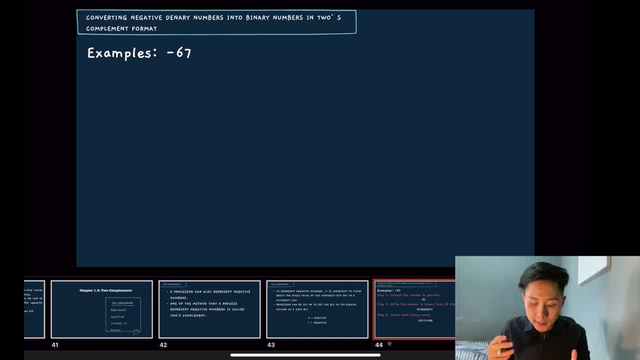 how we convert this, which I believe this is a new syllabus in IJCSC, computer science. it doesn't appear in a lot of passive papers, so do pay attention when you're learning this. so there are four steps that involve in converting this denary: negative denary. 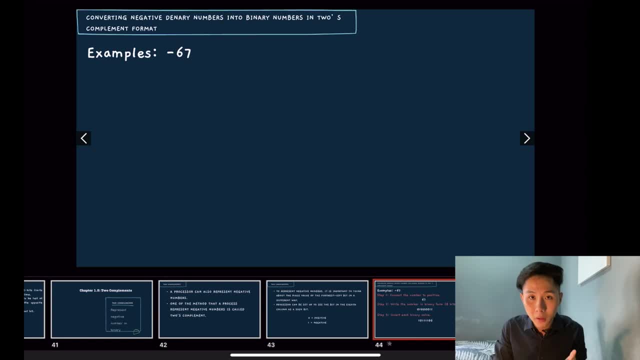 value into two's complement. so first of all, we just have to convert this value number into positive, so negative 67. we just have to convert it into the value of 67. and step 2 we have to write the number of positive numbers into positive numbers. so negative 67. we just have to convert it into the value of 67. and step 2 we have to write the number. 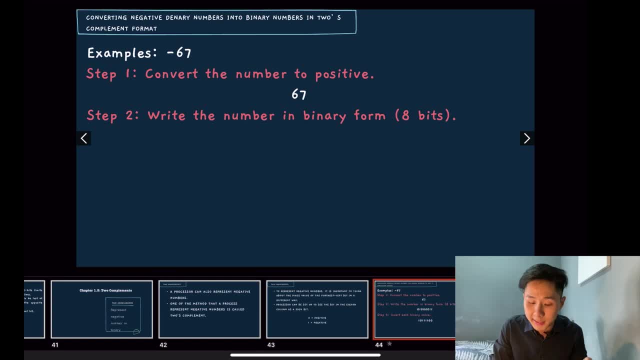 in binary form. what is the binary number of 67? so just to revise, this is how we do this. we keep dividing it by 2 and we get the remainder 33. we got the remainder of 1, all right. so 33 divided by 2, we get 16 and remainder of 1 and do. 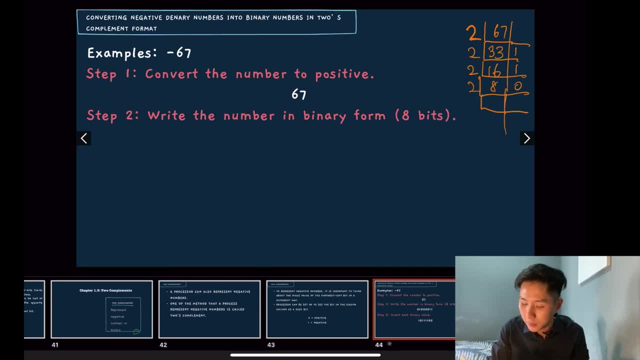 it again and again, until until we divide number 2, until the quotient here becomes 0. okay, so 2 divided by 2, we got 1, 0. that's the remainder. 1 divided by 2, quotient becomes 0 and 1. so our binary value. 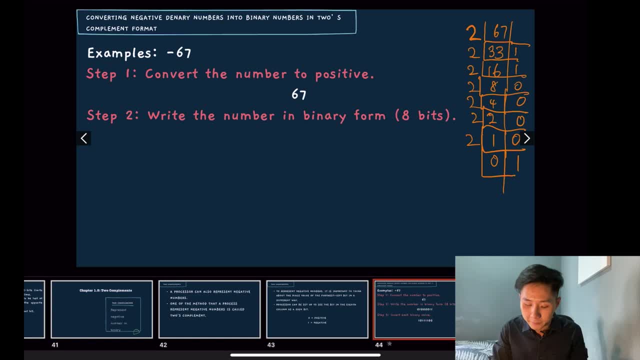 should be 1, 0, 0, 0 0, 1, 1. so this is how we can do this. so one catch here is that if you were to do this, remember if your binary value is 7 digits, remember to add the leading 0. this is very important for 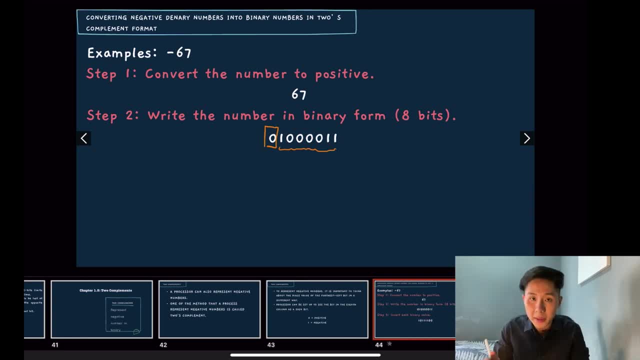 us to find the two complements of this binary value. remember to add the leading 0 if your result is less than 8 bits. so, having calculated this values, the next step is to invert each binary value in which we change 1 into 0 and 0 into 1. so, 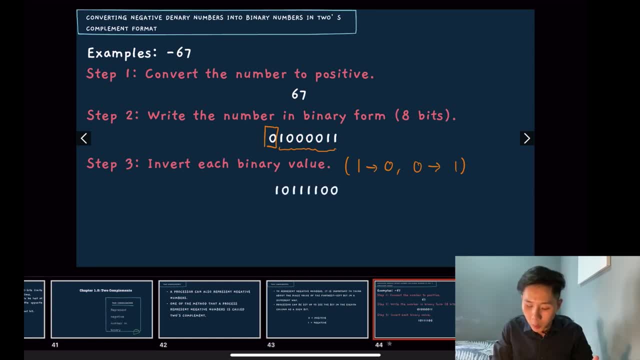 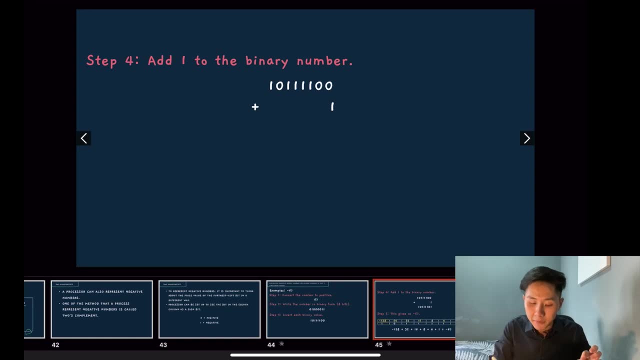 0 to 1. so we got 1 0 1 1 1 1 0 0. we are basically inverting the binary digits and instead of step force by using the inverted value, we add this binary number by 1 and we'll have the. 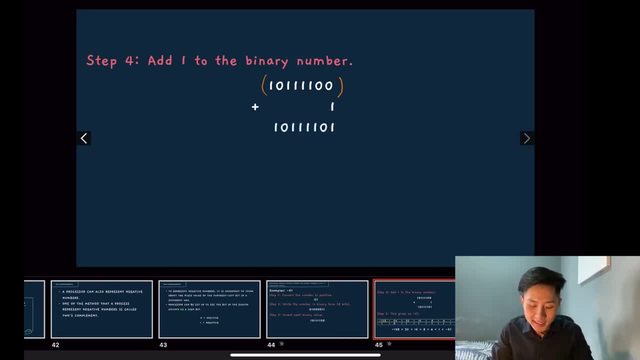 result of 1 0 1, 1, 1, 1 0, 1, and that's the end of our calculation. we have gotten the 2's complement of negative 67, so this is our final result. okay, so let's try to convert another value set like: 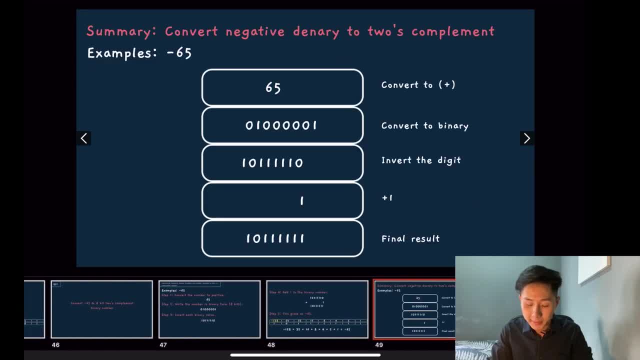 65. you can try it yourself. right, this is how we do this. the four step summary. we convert the value into positive, we obtain the binary number, we invert the digits, we mount, we plus 1 and eventually we get our final result. okay, the five steps that we have. so let us try to do. 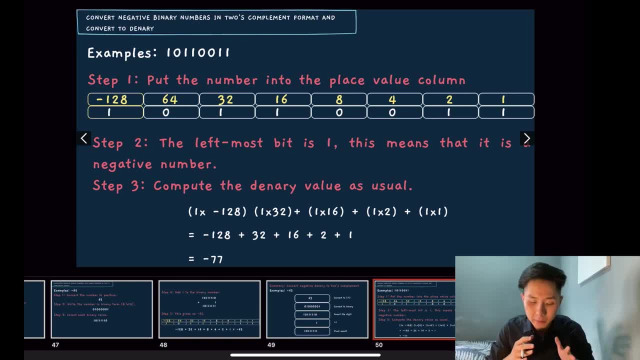 things the other way around. let's try to convert this 2's complement value into a negative denary. so, without having to calculate everything, you would have known that this value here is a negative value. negative value, the reason is because the leading digits of this 2's complement is 1 and. 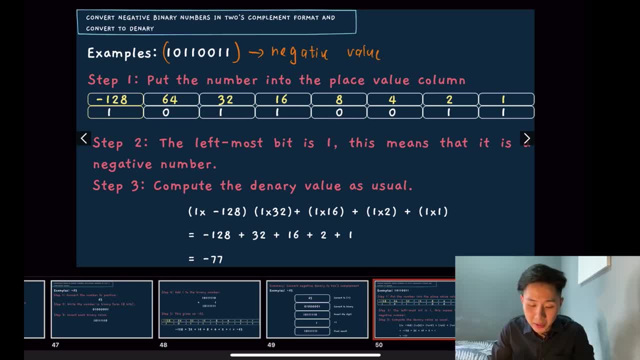 how we do this is very similar to how we convert binary to denary, with one catch is that the place value of the less move value instead of what negative 128 is, it's instead of 128. sorry, it's negative 128 and which we can just multiply the. 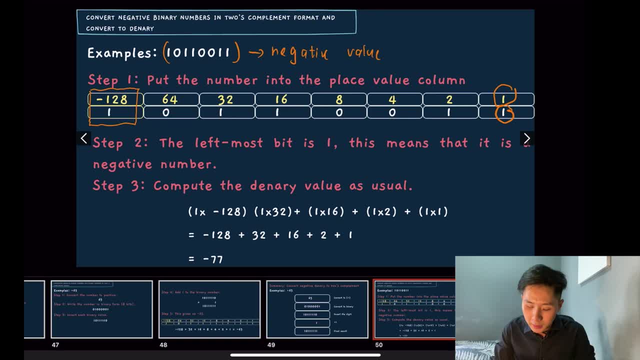 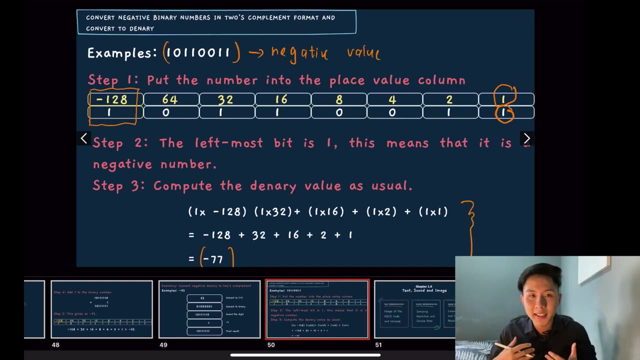 digits value here with the place value and sum them all up together: alright, so that's how it is done when we convert and this is how we obtain the negative denary. alright, so that's how we can represent negative value and binary into a compliment and how we can do things. 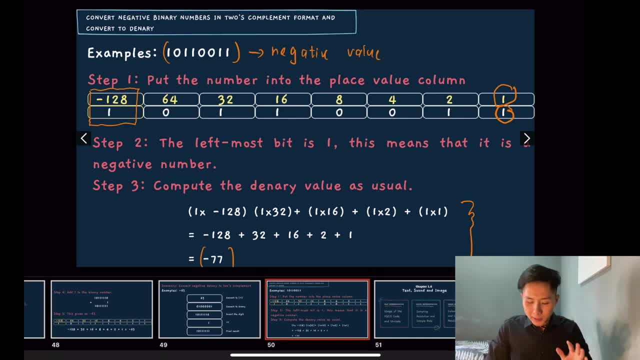 the other way around. okay, so that's our So far. we have learned how to convert different numbers into binary, into a value that computer can understand, but we know that computer can receive data not just in numbers, but also in other formats, such as text, images and sound. 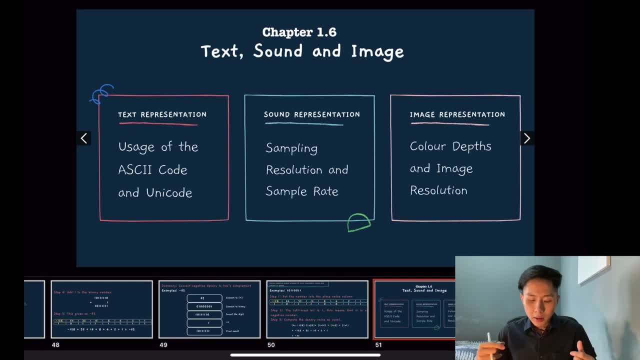 So the next topic that we have here is: how do we represent text, sound and images if the computer can only understand binary? How do we encode this information into a language that into the only language the computer can understand? Let's start off so. that's how we will see all these components, let's say in a game. 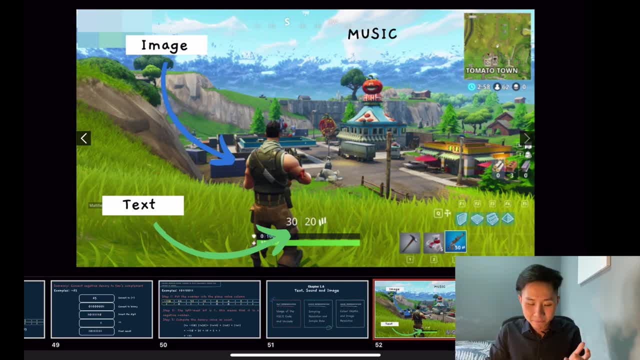 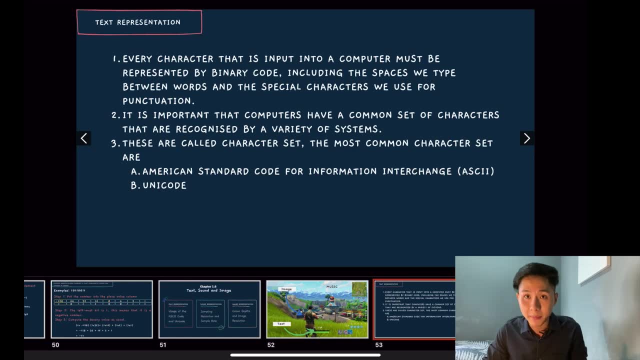 called Fortnite. we have images, text and music, So let's start off with text Here. they say that every character that is input into a computer must be represented by binary code, which means every character that you are seeing now on YouTube on your 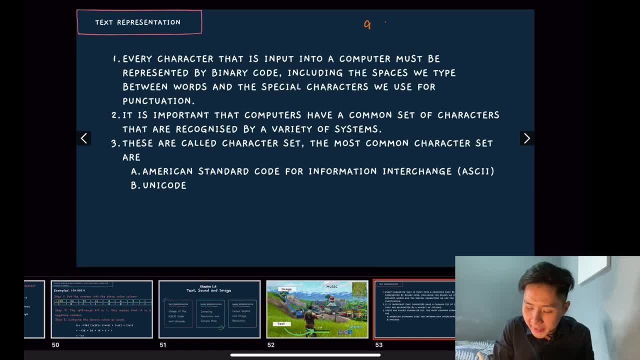 Google Play on your Facebook, on your Instagram, on your Twitter, on your Instagram, on your Google Word, such as A, B, C, D. they are represented by some mysterious, I would say, binary code, even including the space and punctuation that we type in. 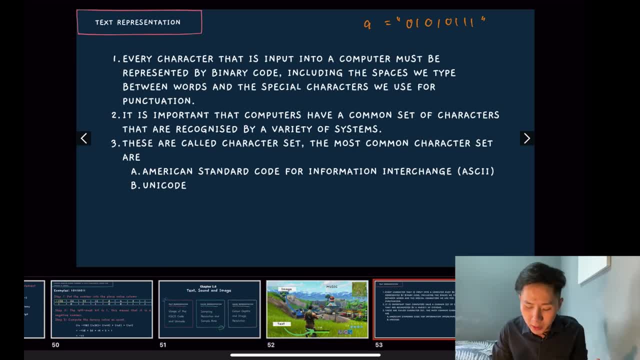 Therefore it is important they say- point number two- that computers have a common set of characters that are recognized by a variety of systems, Which means, given a binary like 1010,, 1000,, the computer has to understand that this bunch. 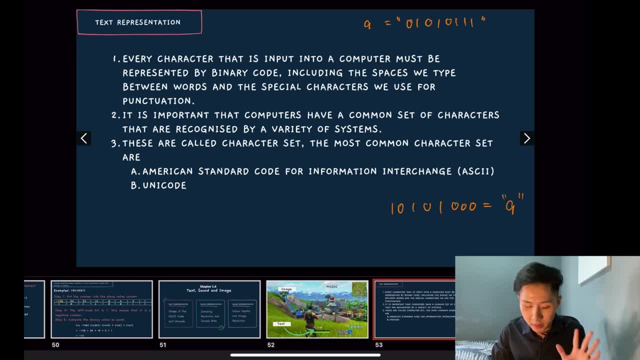 of code is a binary, So the binary code represents a character, let's say A, all right, So the method that we use to map binary into character is called the character sets, And the two character sets that we will learn is, firstly, it's called the ASCII code and 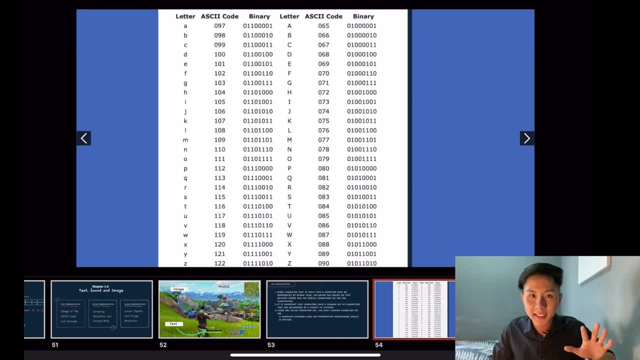 the second one is called Unicode, So let us look at these images here. It is the ASCII code table, in which you can see that each letter here, each letter here, is represented by certain binary. For instance, the binary 01100001 represents the character A. 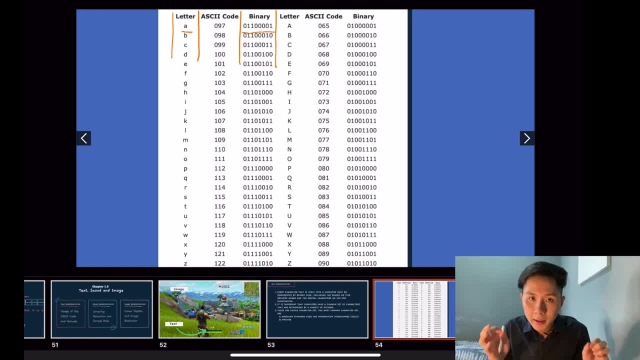 So now, so on and so forth, and by using this method, the computer can understand. okay, the character that we are typing is called A, because it can reach the binary in 01100001,. okay, So that's how a computer can read text. 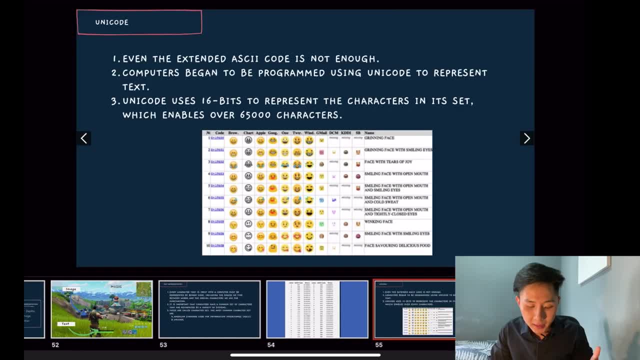 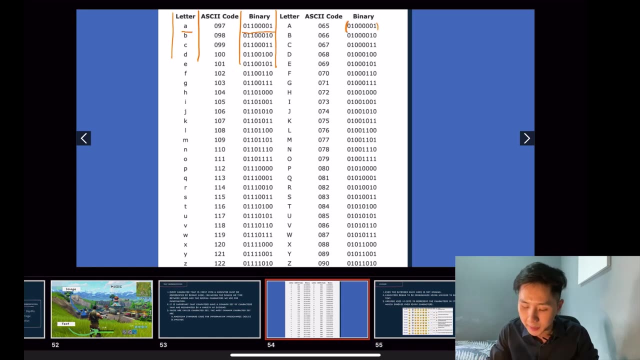 This is called the ASCII code, The other methods, the other character sets that they are commonly used nowadays called the Unicode. and this is because the extended the ASCII code is not enough. If you look here, we only have 8 bits here. okay. 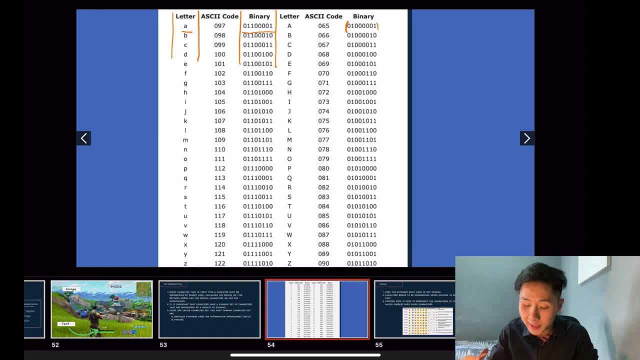 We know that the number of representation a 8-bit binary can have is there's a limit to it. It's only 225 characters, Which means ASCII code can only adapt to 255 unique characters. But we know that as we will type different languages into our computer, such as French, 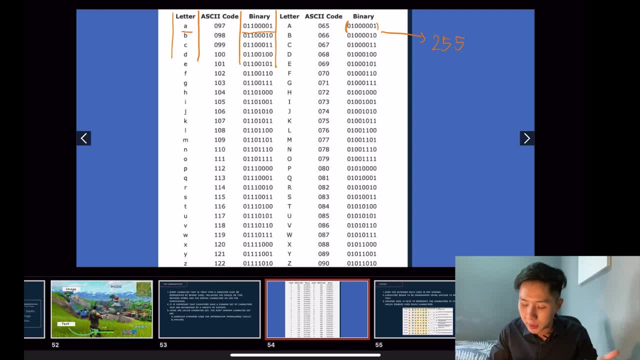 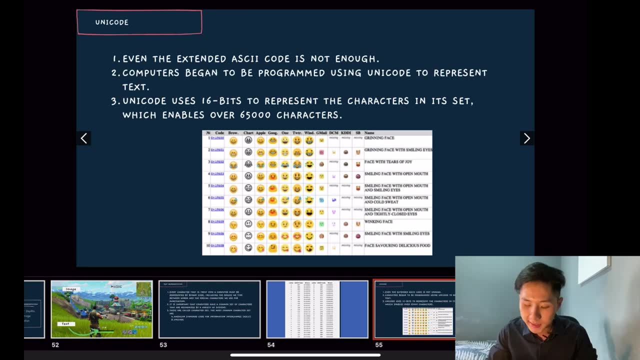 Mandarin. we need more characters. we need more digits. So that's why Unicode is invented: It uses 16 bits instead of 8 bits to represent characters in its set, which enables over 65000s of characters, And these characters can be the emoji that we use day to day. okay, 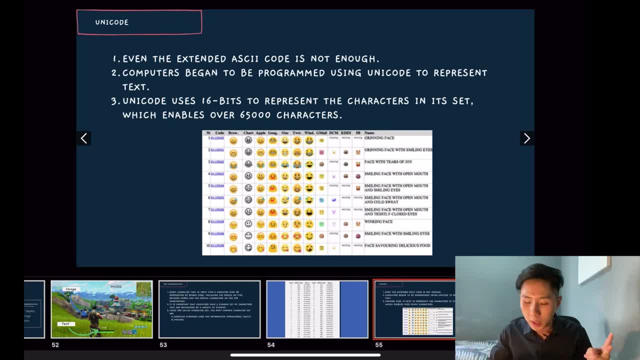 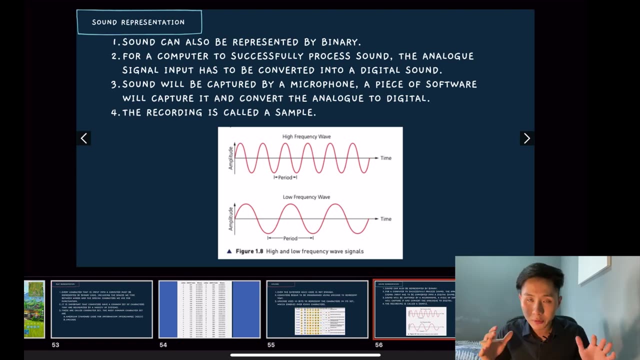 So the two ways that we learned here, which a computer uses to represent text, is called firstly the ASCII code And also the unicode. So let's move on to sound. and they say here: sound can also be represented in binary. The voice that you are listening, now my volume, they can also be represented in binary. 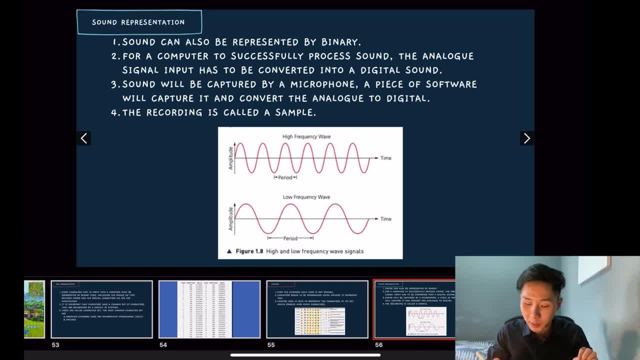 And the way they do it for a computer is they experiment with text and Knight mode to know if it has nodes and pincers. So you say, hey, I'm all set successfully process sound. the analog signal input has to be converted into a 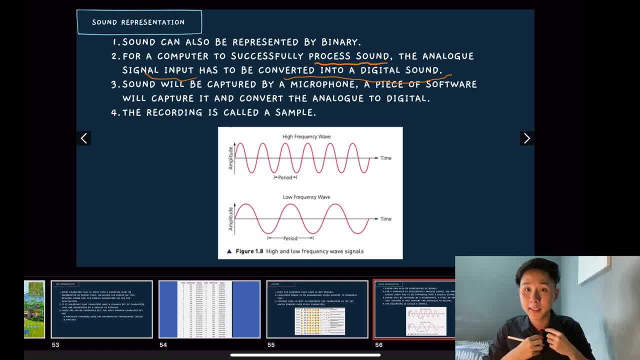 digital sound. sound will be captured. for instance, it will be captured by a microphone here that I have and a piece of software will then capture it and convert this sound into digital. digital data means zero and one, and this recording. this is the first keyword that we look into. it's called a sample, the. 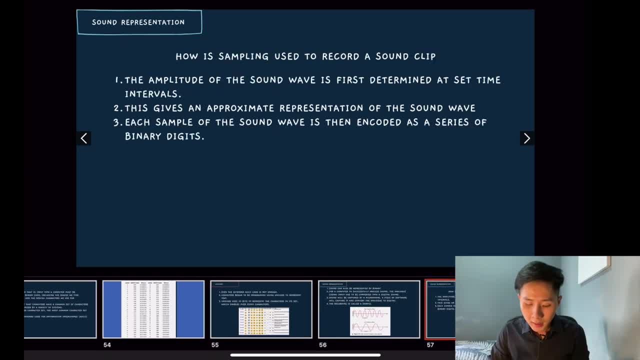 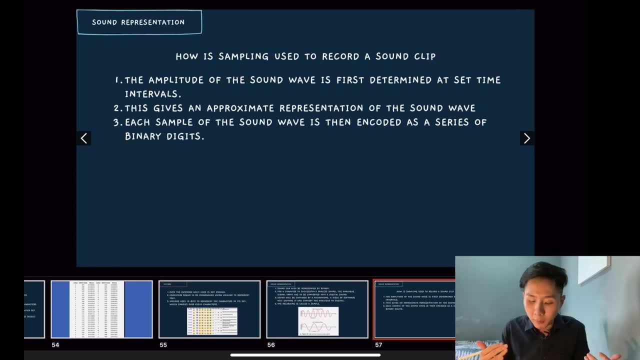 voice that they record is called a sample, and how sampling is used to produce a clip. so this. these are the three steps. first of all, the amplitude- how loud my voice is- is determined at set intervals. this gives an approximate representation of the sound wave, and each sample of the sound wave is then 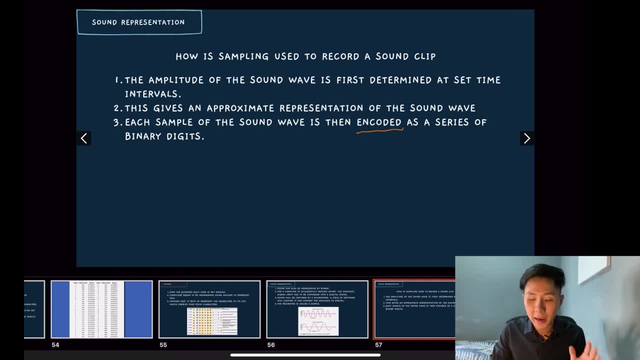 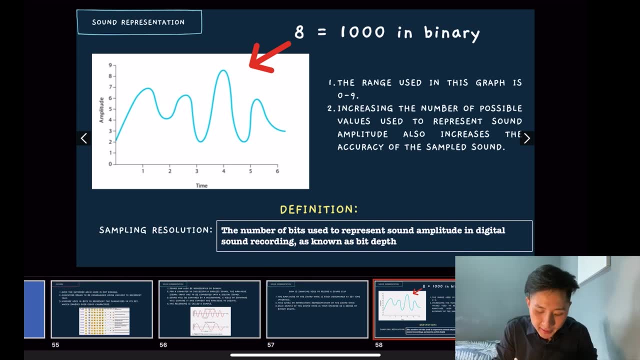 encoded the keyword as a series of binary digits. for instance here we have a sound graph here which record how loud the voice is at a particular time. so one, two, three, four, five, six, and each in time interval, the amplitude will be quantified. so the range that is used in this craft is from: 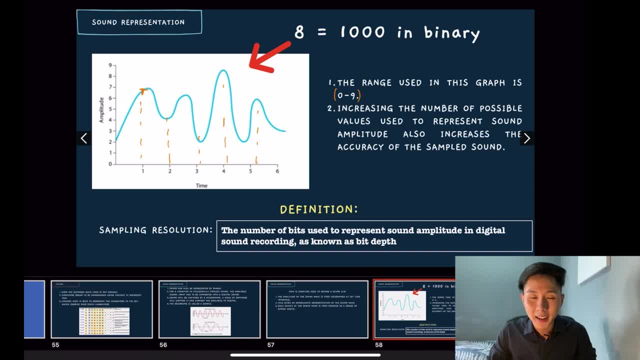 zero to nine. so we know that zero and nine can be encoded into binary. so that's how computer can read sound. and this, if I will. in point number two they said that if we were to increase the number of possible value use, so instead of zero to nine, if I were to increase 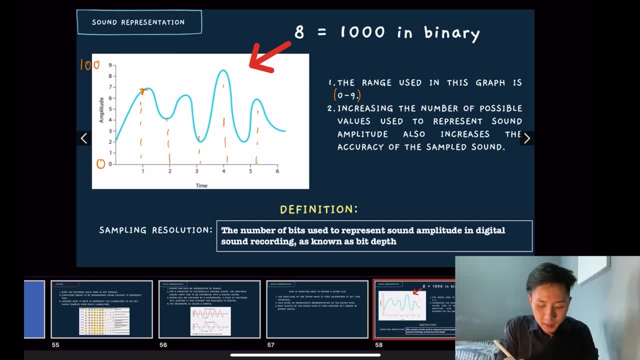 this into zero and one thousand, which means I, and long elongates the range. this will increase the accuracy of the sample song because the range is bigger now. but everything comes at a cost. if I were to record, if I were to increase the range, this means that the number of bits used to represent 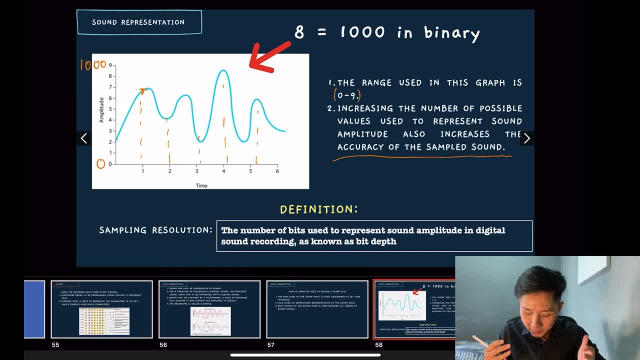 this sound will have to be increased. so this is called the sampling resolution, in which it is the number of bits- here you have to remember this definition- the number of bits used to represent sound amplitude in digital sound rate recording, which also known as beat that, beat that. that's the equivalent of 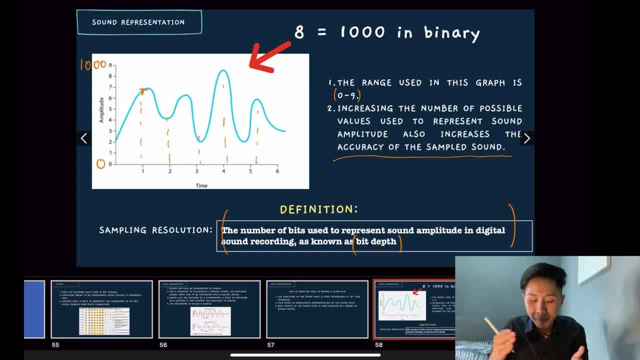 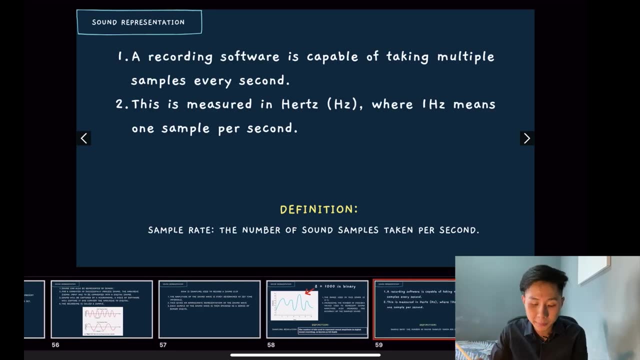 sampling resolution. in other words, if you were to increase sampling resolution, you increase the accuracy of the song, which means your sound will be of greater quality. so that's how sound is represented, and recording software here is also capable of taking multiple samples every second. this is measured in 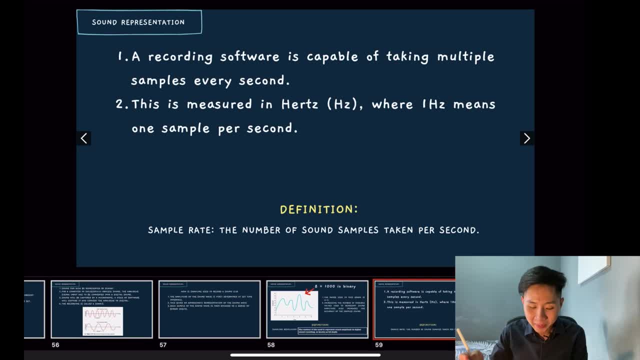 Hertz, where one Hertz means one cent per second. all right, if I were to record my sound in, I want three samples per second, it would be three Hertz. so that's here's another definition here, called the sample rate, then, which is called the number of sound samples taken per second. all right, 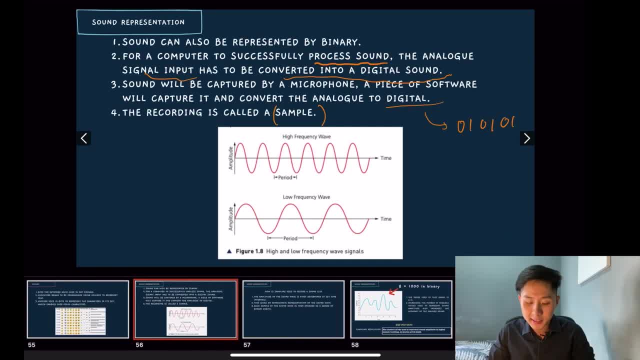 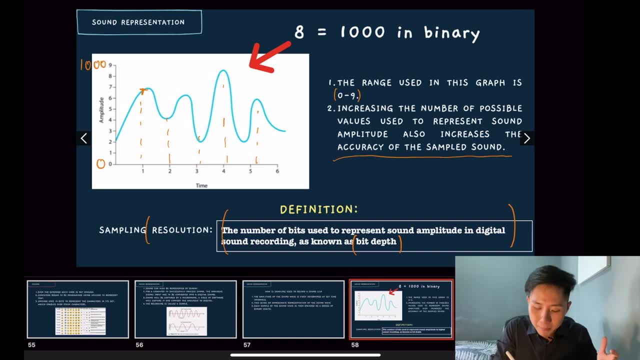 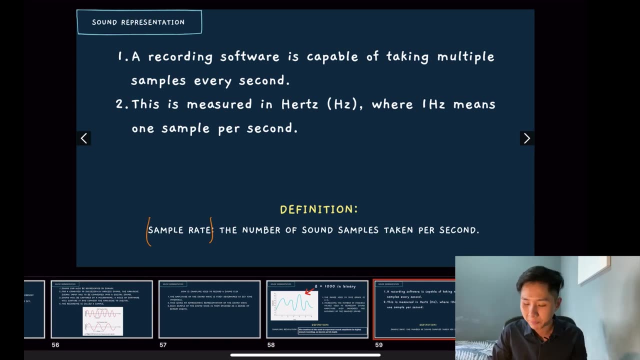 so that's all about sound. the tree definition that we have here is firstly the sample, second one the sampling resolution. what is the number of bits used to represent the amplitude of my sound? right, the one is the sample rate. how many sample do I take per second? and here are the pros and cons of using a. 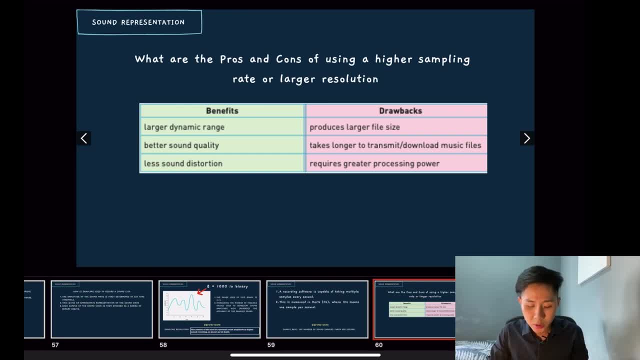 higher sampling rate or larger resolution, which is if I were to use more bits to represent the amplitude. of course the size of it will be bigger, produce larger file size, but it will also have larger dynamic range, better sound quality, less distortion, and the drawbacks of it is: 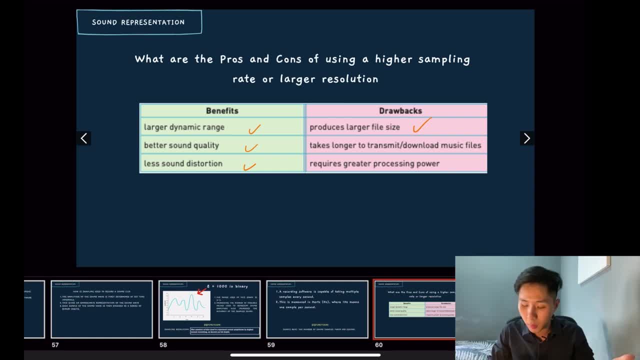 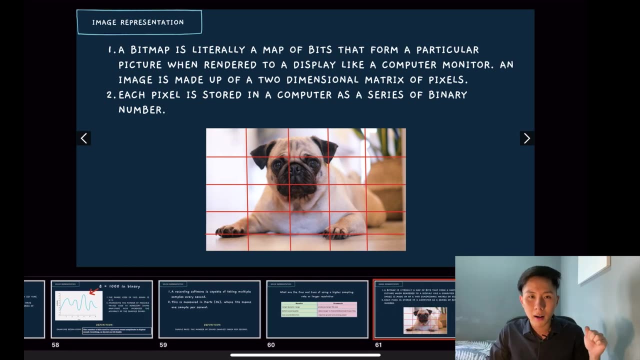 larger file. it takes longer to download the file and requires greater processing power. and it is a very commonly asked question in the exam. so make sure you understand all this benefits and drawbacks so that you can evaluate accordingly in your exam. okay, so next up. having talked about how computer 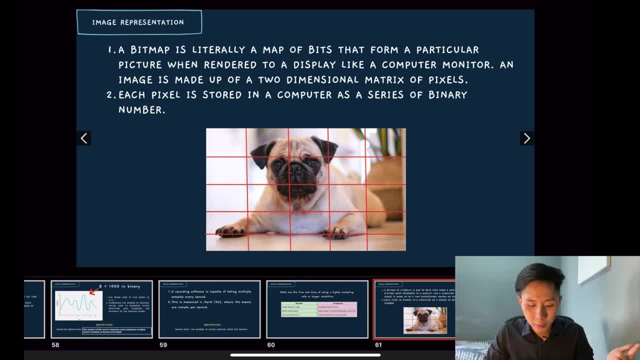 represent text, how they represent the sound quality and how they represent the sound quality. so next up, having talked about how computer represent text, how they represent sound, will move on to image. image. every image that you see now, even the video that you are seeing now, is actually represented in something called a bitmap. 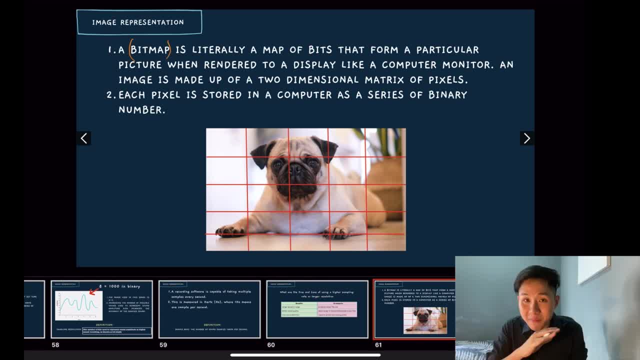 a bitmap, which is literally a map of bits that forms a particular picture. video is just a series of pictures and, when rendered to display like a computer monitor, an image is made up of two dimensional- the horizontal axis and the vertical axis- and each pixel is stored in the computer as a series of 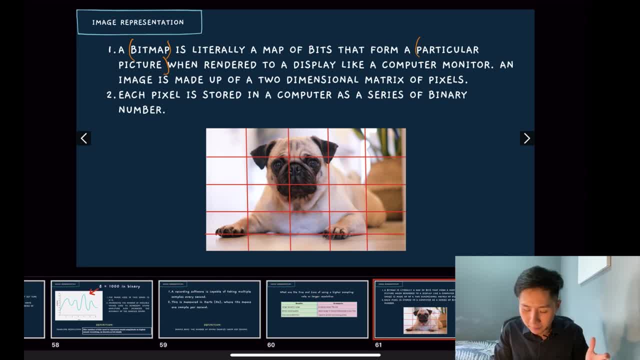 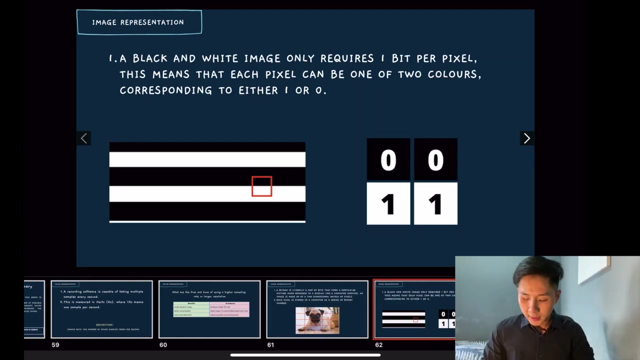 binary numbers, and here we have a very cute puppy, and this image is also represented in pixel. to simplify it, I draw a five to five pixel here. so this is: they have five vertical bar and five horizontal bar. so this is a five to five image. okay, so let us look at some of the image. so 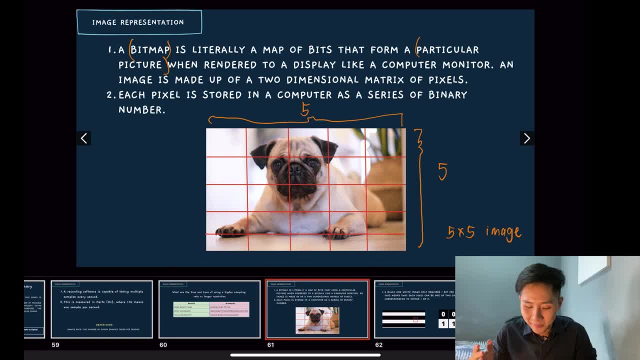 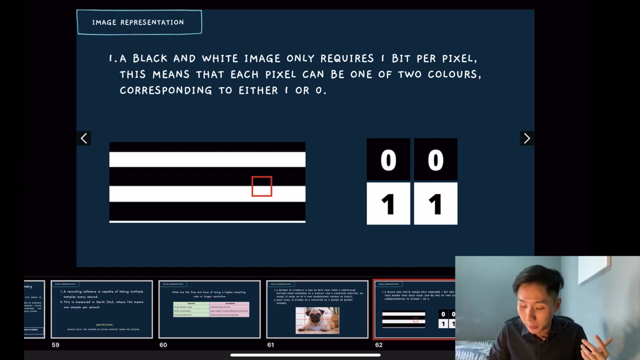 as I said, computers can only understand binary. so this means that each pixel here they are actually just a bunch of binary value, they're just a binary route in which each binary value here represent one color. okay, so here we have. so imagine that here I only use two digits, only use- sorry- one bit to. 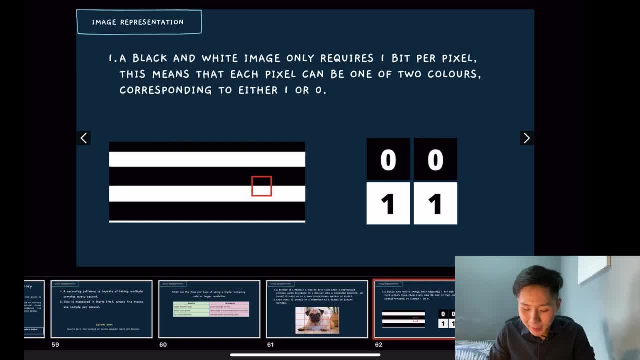 represent one pixel. this means that my image can only believe black and white, because if I only have one digits, the value that I can have is either 0 or 1. it can be either 0 or 1. that means I can only have black and white, which means if this pixel is called is 0, has the value of 0. 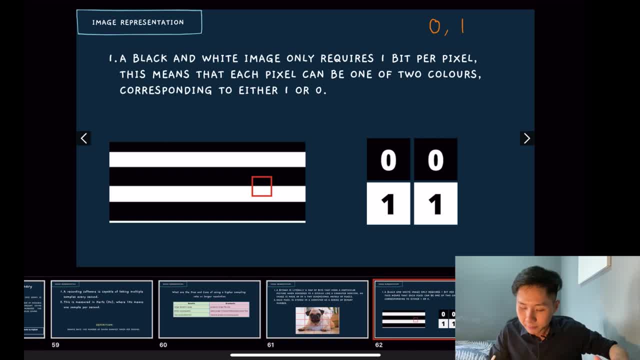 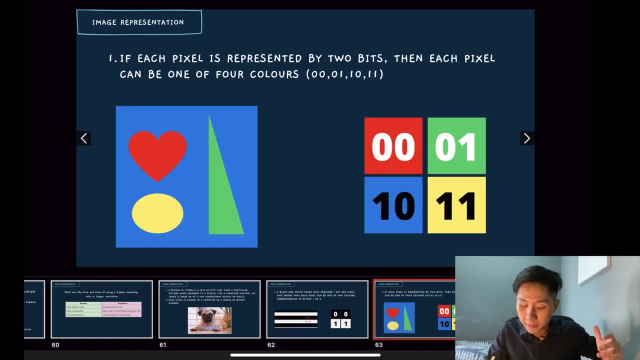 the computer will represent it in black color. however, if I were to increase the number of bits used in each pixel, let's see if I were to increase it. so imagine if I use two pixels- I mean two bits in one pixel- I would have four possible values: 0 0 0, 1, 1 0, 1 1- and I can assign: 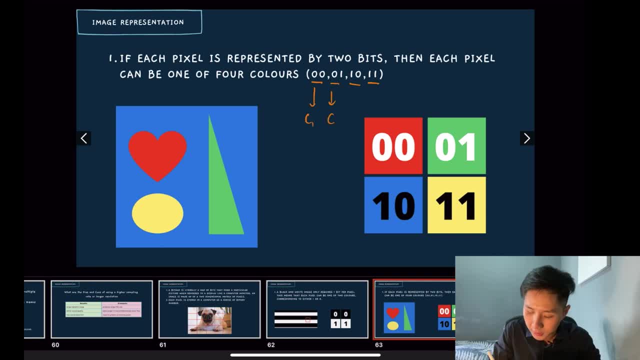 each code here into one unique color color: one color, two color tree colorful. which means if number of bits that I use to represent one pixel is 2 bits, I can have an image in delta four colors. so as you can see in this image, there are four colors here: one, two, three, four. so the number of bits 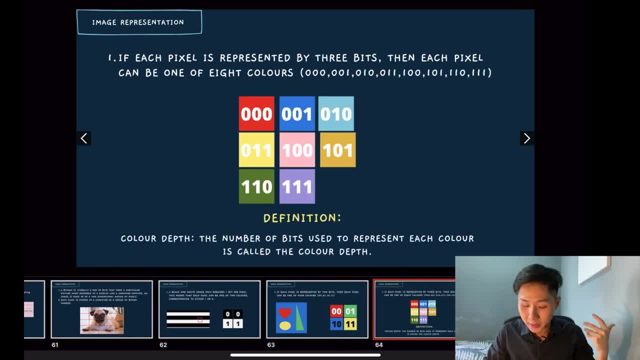 used to represent each pixel is only two bits, and if I have to increase it to three bits I would have eight colors, and here I will introduce a new terminology which is called the color depth. the color depth is the number of bits used to represent each sorry, each color, each, yeah, each color called. it's called the. 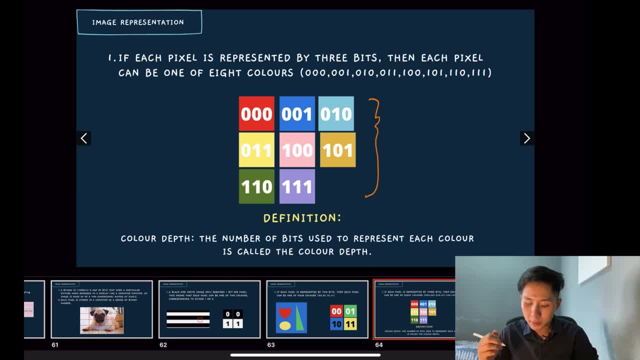 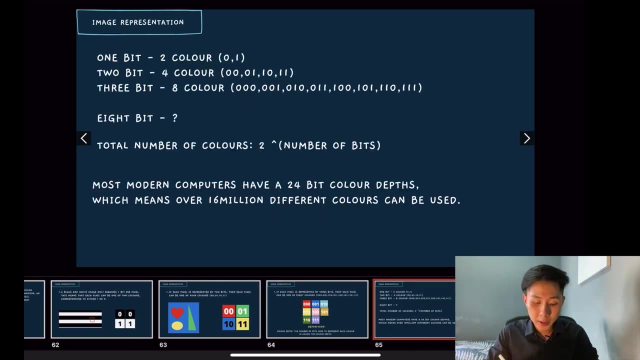 color depth. so in this image here, if I were to use three bits to represent each color, my bit, my color depth will be equal to three, two, three. so so, like what we see, if I only use, if my color depth is one bit, I would only have two colors. if I have two bits might have two, four. 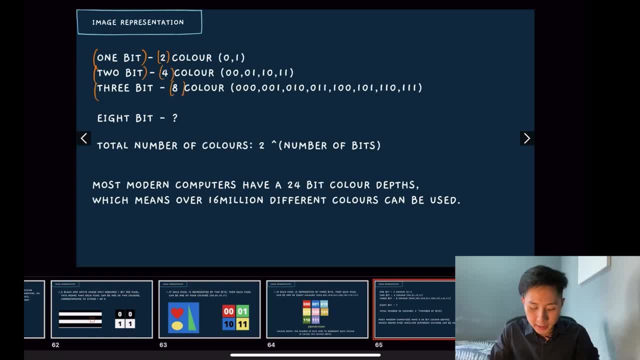 colors, three, eight. so what about eight bits? right, we need a formula to calculate it, and the formula that we can use to calculate the number of colors we have is two to the Perry plus three by power of number of bits. If I have two bits here, or use two to the power of two, as you, 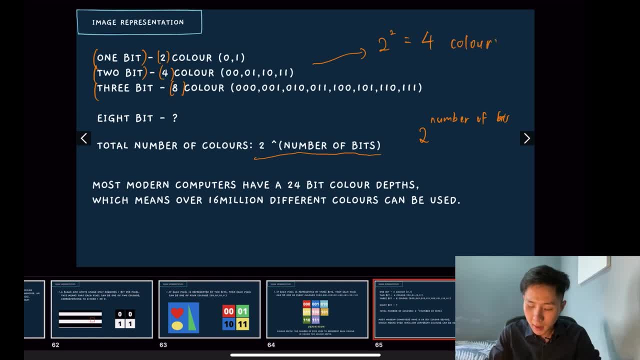 can see, I would have four colors. However, in modern computers that we are using now, they usually have 24 bits color depth, which means they can produce over 16 million different colors. That's how a computer can produce a variety of colors. That's image. 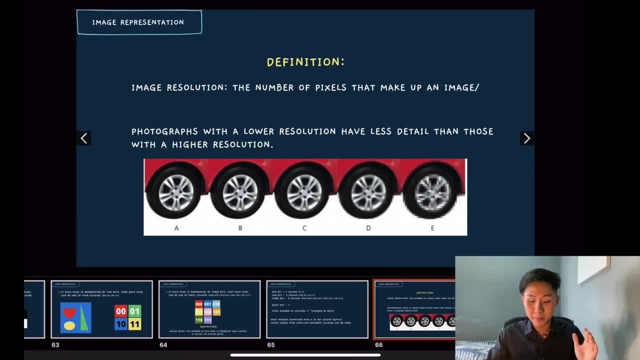 Another term that can affect the quality of an image is called an image resolution, which is the number of pixels that makes up an image. Try to look at this diagram from A to E- The rightmost image here- it has the least resolution, which means the number of pixels, number of. 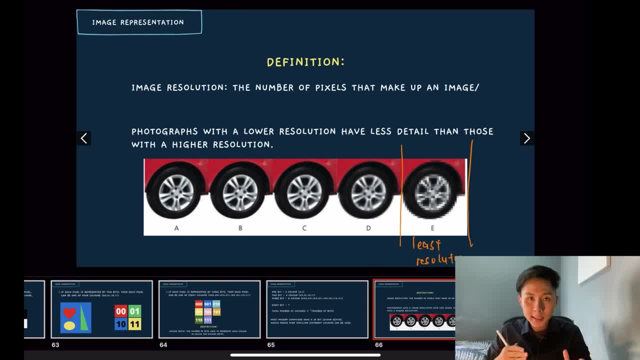 boxes that form the image is the least. This is why it has the lowest quality. However, if you look at the leftmost images, it is the clearest b because it will have a higher image resolution, more pixel to represent that image. 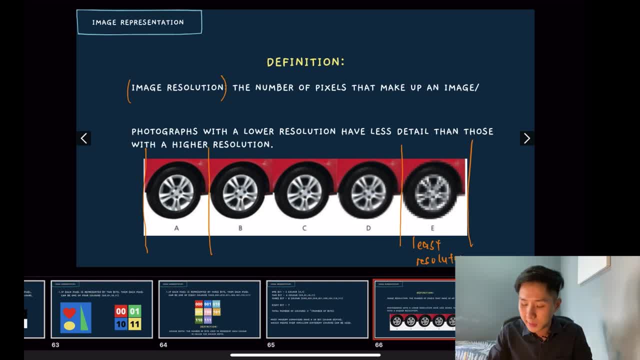 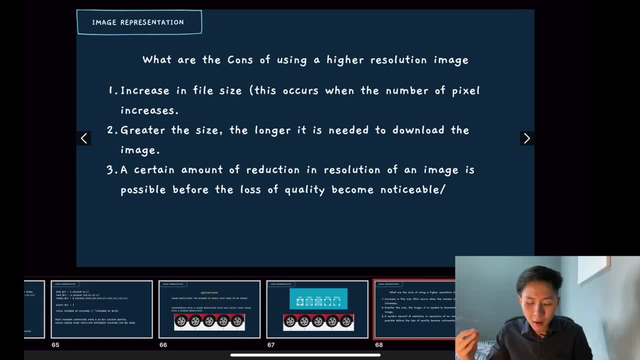 So this is the definition of image resolution: the number of pixels that make up an image. So another picture here. So again they asked: what are the cons of using a high resolution image? What if I want to have a higher quality image? 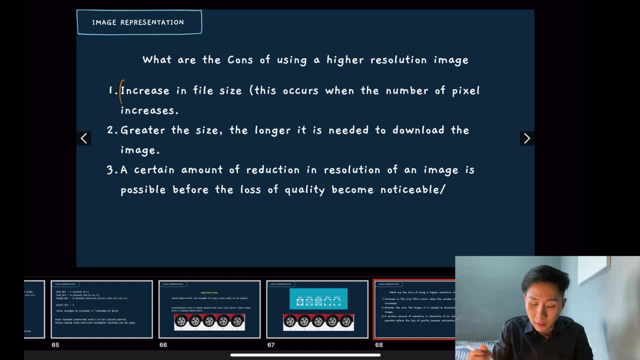 This is pretty common sense, which the first one is the increase of file size, because the more pixel that you have, the more binary bits that you will need to store, And greater the size, the longer it is to download the image. And then point number three, 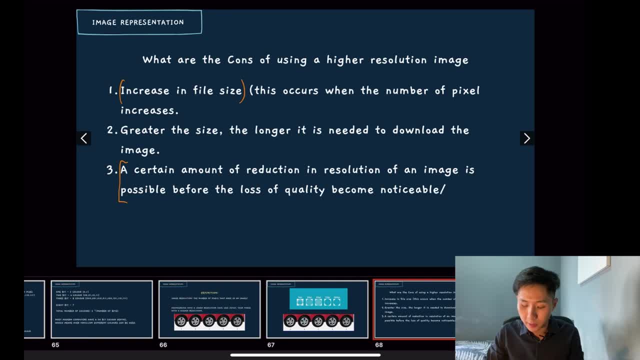 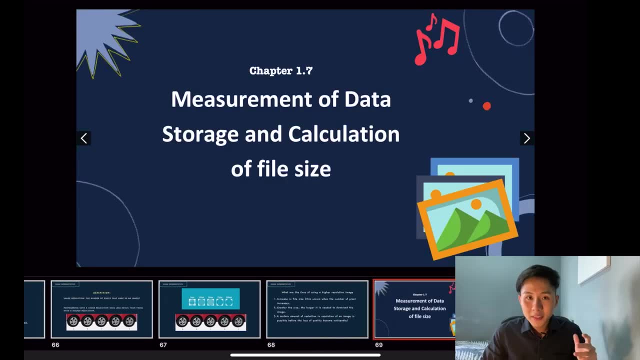 a certain amount of reduction in resolution is possible before the loss of quality become noticeable, which we will touch more of this in data compression. So now we'll move on to how we measure the size of certain data in computer. How does computer measure how many gigabytes, kilobytes, that a file has? 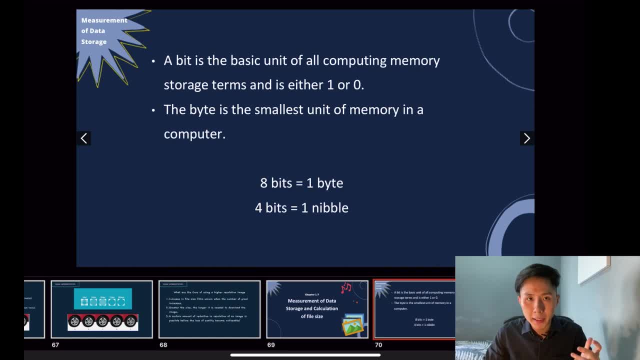 So we're going to talk about the size of certain data in computer. How does computer measure how many gigabytes, kilobytes, that a file has? So let me first learn some of the basic terminology of storage in computer science. The first one is called the bit. 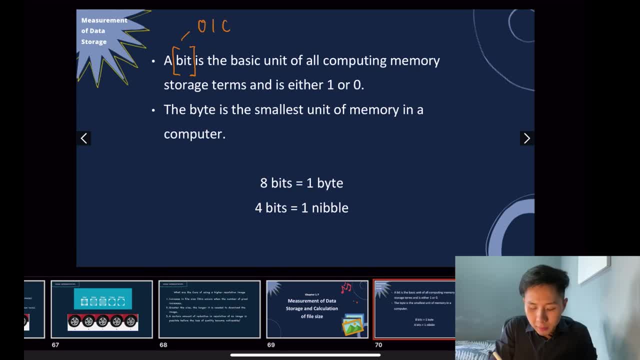 The bit, which is zero and one. So this is how computer stores data. It is the basic unit of all computing memory storage term, and it's either zero or one. And move on. we have the terminology of byte. It's the smallest unit of memory in a computer. 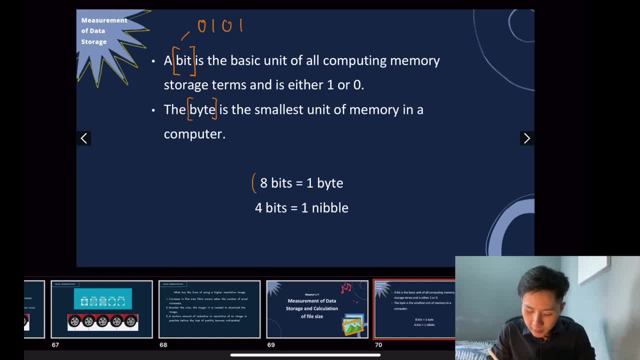 which every eight bits here, like you see here, is called one byte, one byte. So if I were to have zero, one, one, zero, one, one, zero, zero stored in my computer, my computer will calculate this as one byte. 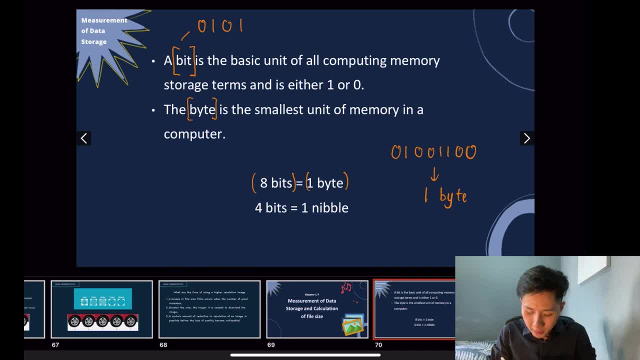 because it's equivalent to eight bits. And another terminology that you have to remember is called the nibble, which is half a byte. four bits, all right. So that's the basic terminology, But we know that computer can store a lot of bits. 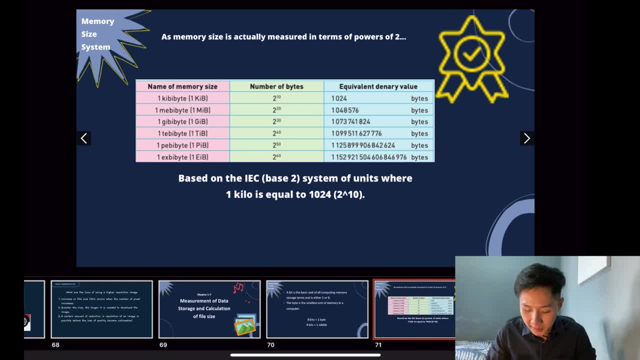 Therefore, a better organization system is needed, which we will learn is called the IEC base two system of units, where one kilo is equal to two to the power of 10 bytes, which is equivalent to 10, 1,024 bytes. 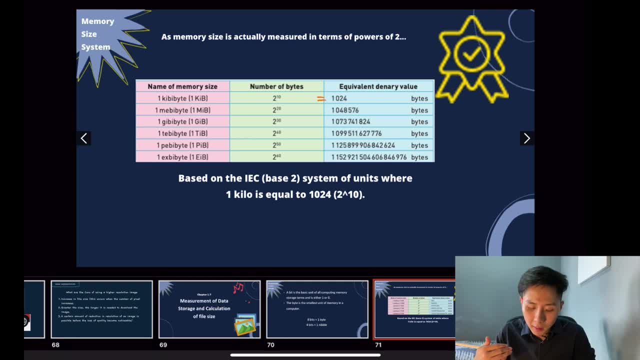 So by using this we can name the bytes better. Instead of saying I have 1,048,500 bytes, I can just say the size of it is one mebibyte. It's easier to visualize and also easier to pronounce it. all right. 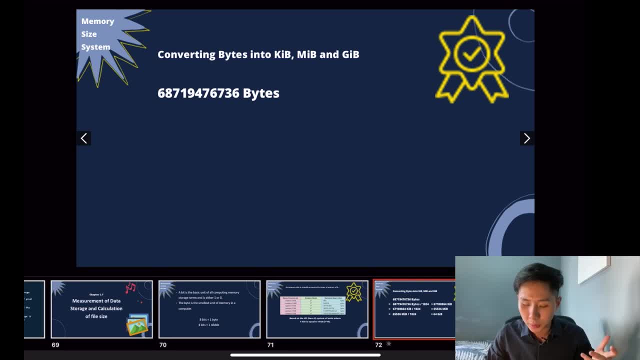 So let us try to convert this bytes into kibibyte, mebibyte and gibibyte. The way we do this is very simple. First of all, if I were to convert bytes into kibibyte, I would just have to divide this value by 1,024.. 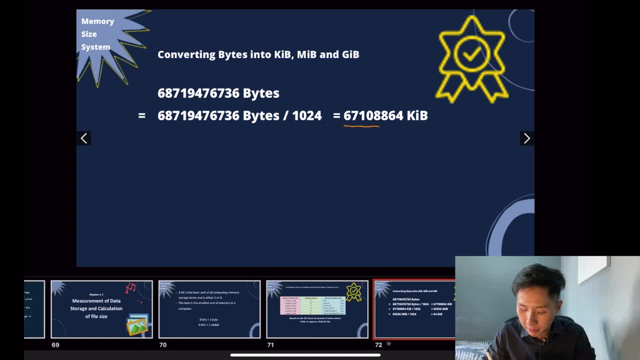 And the value that I have here will be the value in kibibyte. What if I wanted to be mebibyte instead? All I can do is just to divide it again by 1,024.. We'll have get the value in mebibyte. 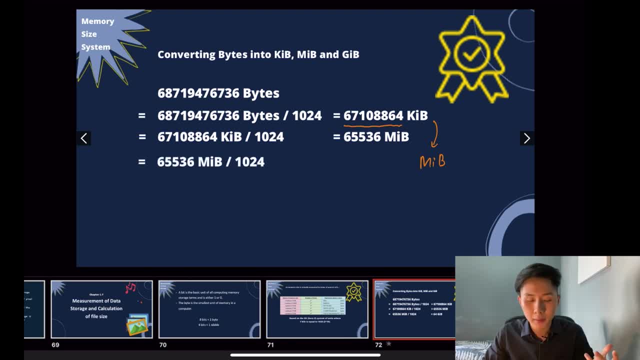 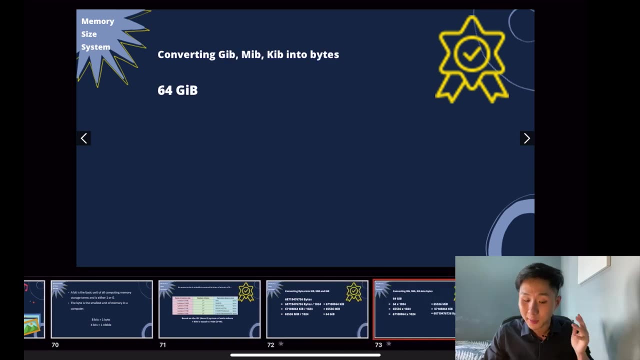 If I want gibibyte, I'll get again divide by 10,024.. I would have 64 kibibyte, All right. So that's how we convert bytes into the different units that we have, And to do this another way around, as you might have already guessed. 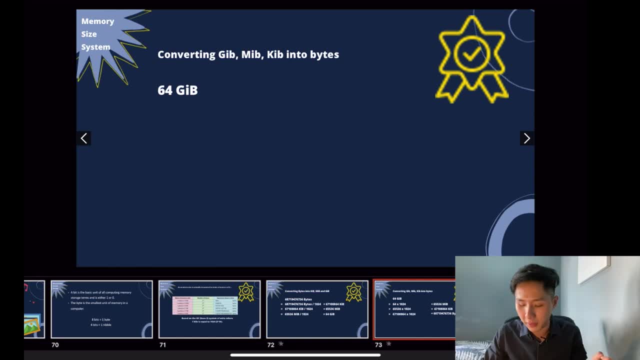 is that we just have to multiply instead of dividing it. Just multiply by 1,024 and get the value. All right. So that's how we restored, how we convert gibibyte to the different units that we have here. Okay, 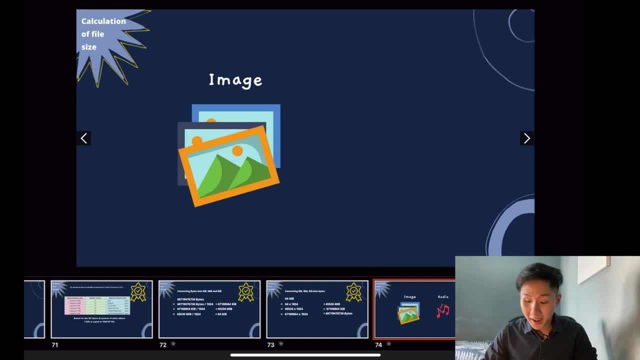 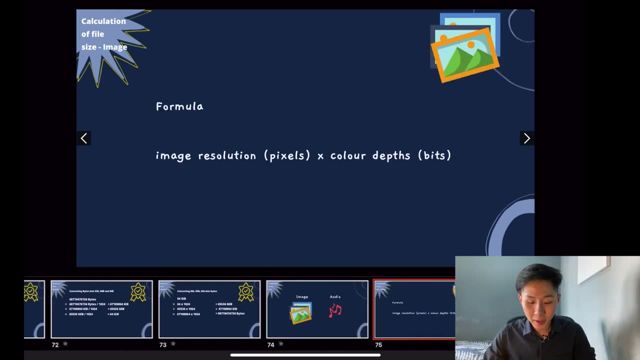 So let's do some exercise which can help us to calculate how big a size an image is, and also audio. So let's start off with image. How do we calculate the size of image? So there is a formula here which is to calculate the size of an image. 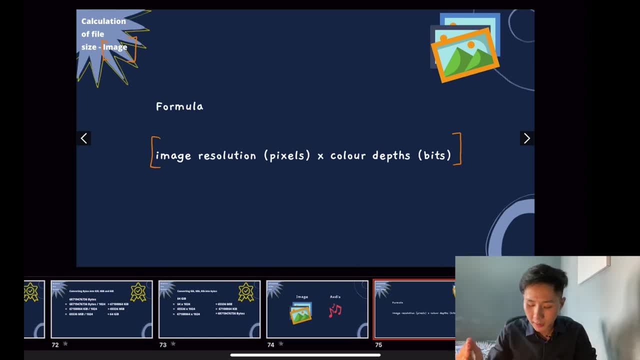 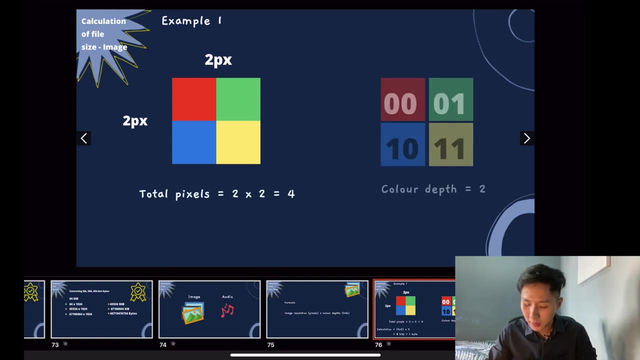 we just have to use the image resolution pixels and multiply it by the color depth, And the way we can derive this formula is very straightforward. So imagine that we have a 2x2 image And we have a color depth of 2.. 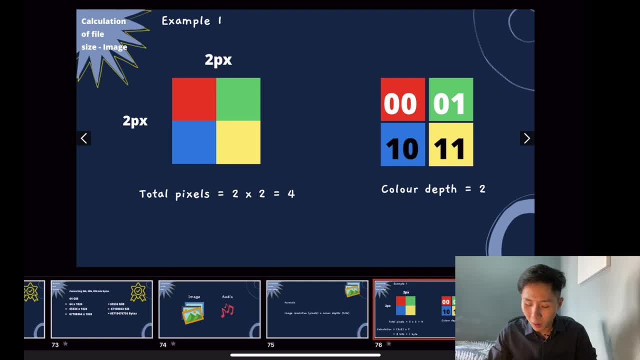 And, as you can see here, the way we can calculate the size of this image is to first determine how many box there are- 1,, 2,, 3 box, Which we can get it by multiplying the image resolution 2x2.. 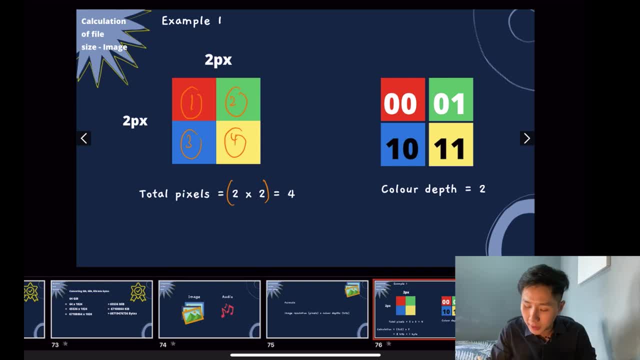 We have 4 boxes And each boxes we need to know how many bits are there in each pixel, And here we have 2.. So the formula is image resolution by color depth. So we are basically calculating how many bits are there in this image. 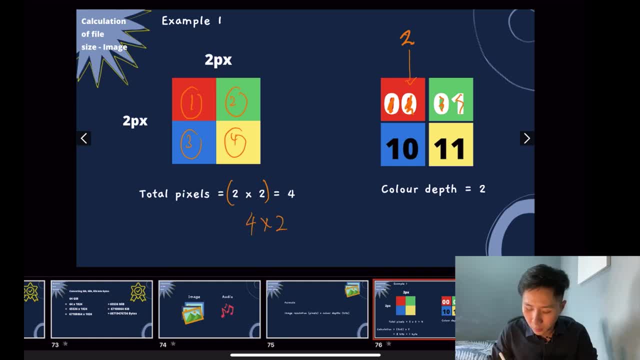 And we can just use 4x2, we'll get 8 bits. So, as you can see, this is the image resolution. Image resolution And this is the color depth And the size of it would be 8 bits. 8 bits, which is 1 byte. 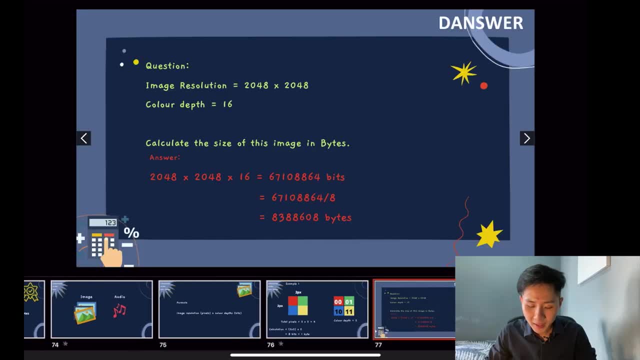 So this image, the size of it is 1 byte. So let's move on to a real exam question: Image resolution. Let's say I have an image of 2048x2048 with a color depth of 16. I can just use the formula. 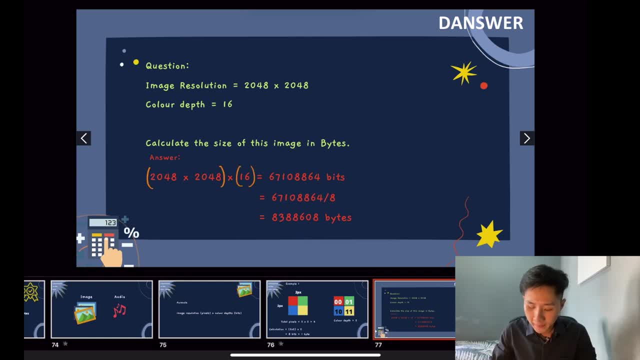 The image resolution multiplied by color size And we'll have gotten the value- the size of it- in bits. But note here: the question said I want the size of this image in bytes. Therefore, one more step is needed here, which is we need to divide by 8. 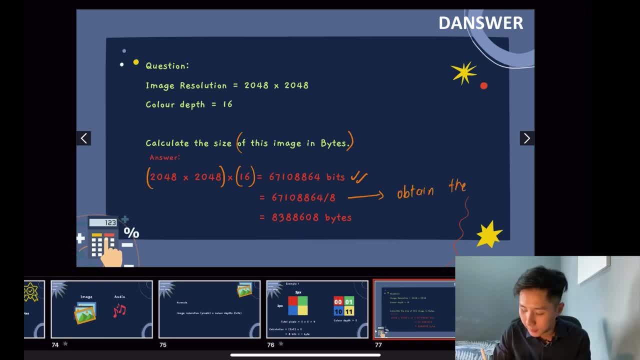 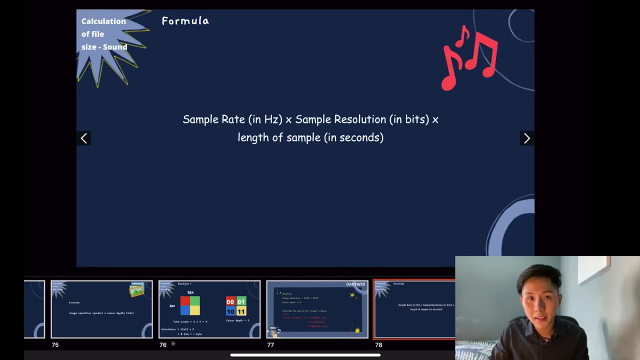 to obtain the storage size in bytes. The storage size in bytes. Okay, so that's how we get our answer. So, so that's how we calculate the size of an image. Alright, it's pretty straightforward, And let's move on to how we calculate the size of a sound. 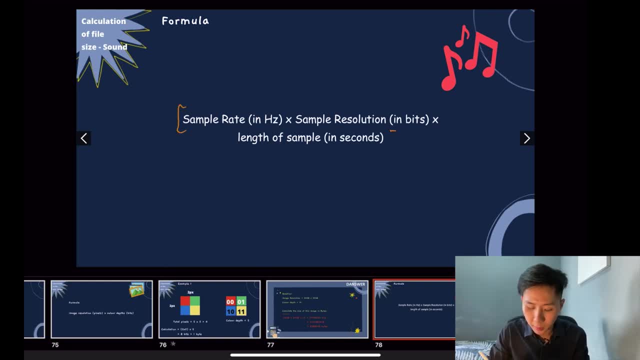 And the way we calculate this is to use this formula. First is that we use the sample rate multiplied by the sample resolution and also the length of sample in second. So let's look at one example question. Imagine that this is the question they said. 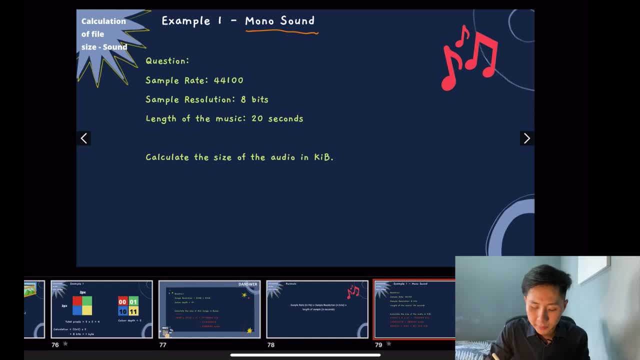 they say that this is a mono sound And they give you some sample rate, sampling resolution and length of this music in second, And they said they want the size of the audio in kibibyte. So let us try to use this formula. 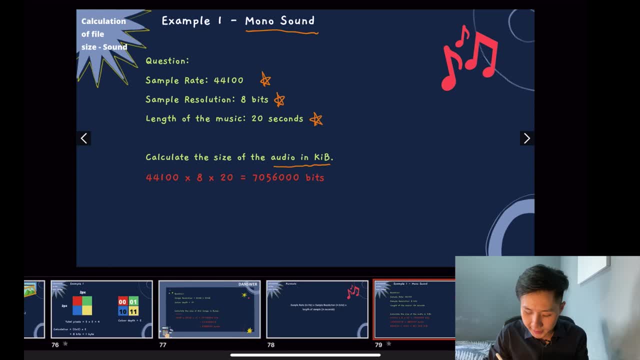 We'll have get gotten 7 million bits. Okay, but since the question says they want the answer in kibibyte, we need to first convert it to byte, And the way we do this is to divide the number of bits by 8. 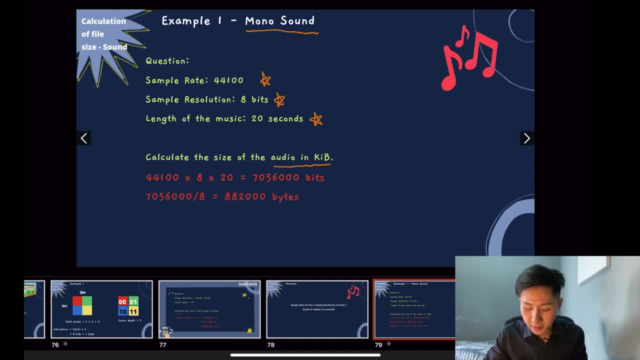 and got the bytes, And to convert bytes into kibibyte we have to divide it by 1024.. So this is how we got the final answer: It's 861 kilobyte kibibyte. So that's. 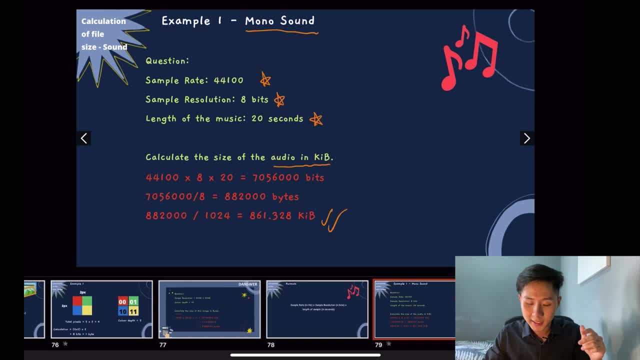 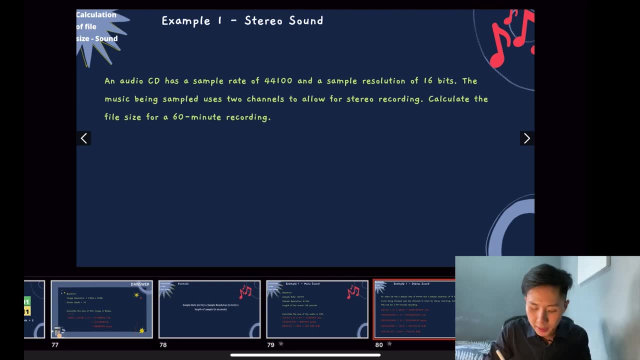 for mono sound. Another question that they might ask is that they will say: here we have a stereo sound, So let's read the question. An audio CD has a sample rate of 4 to 4000.. Let's highlight the important details, alright. 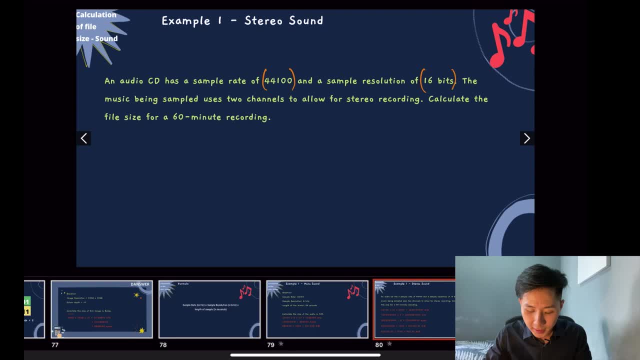 Sampling resolution of 16 bits And the music sample uses two channels to record for stereo recording. Stereo recordings means if you were to bring your headphone, the left and right headphone will have a different voice. That's called stereo recording And calculate the file size. 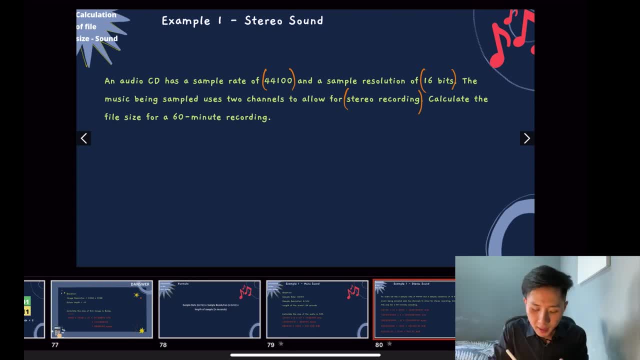 they said for a 16-minute recording. So that's the catch here. Remember: the formula is sample rate multiplied by sampling resolution and multiplied by time, But the time should be in seconds. Therefore we need to convert this length into seconds. 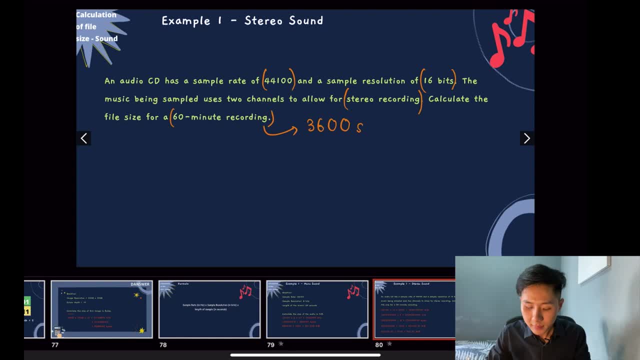 which is 3600 seconds. So here, the way we can do this is just to multiply everything together, alright, 44000, and so on to get the number of bits. But here's the catch here, Because this is a stereo sound. 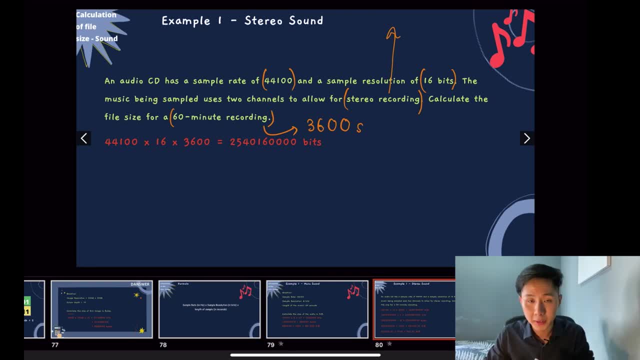 we need to multiply the value that we have here by 2.. So we need to multiply the number of bits by 2.. This is only needed needed for stereo. If it is a mono sound file, it is not needed. Okay. 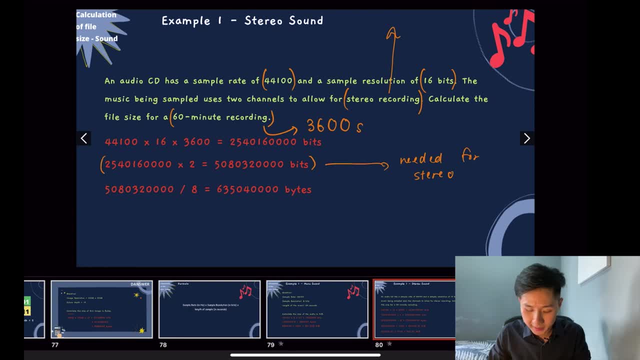 So that's how we just have to divide it by 8 to get the number of bytes And eventually multiply by it to get the file size in, maybe byte. So that's about it for how we calculate file size in images and in sound. 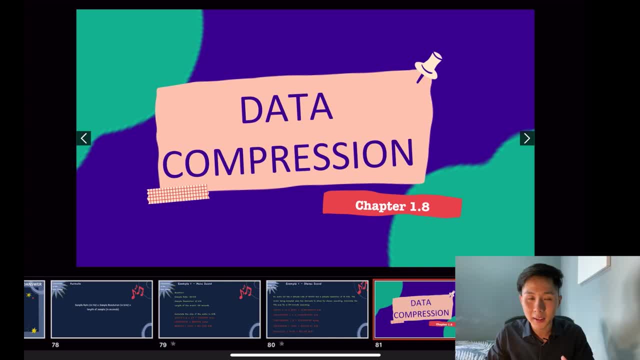 And let's move on to the last topic of this video, called data compression. So, like what we know just now or we see just now, if we want to have a very high quality image or sound, we need to increase the number of bits. 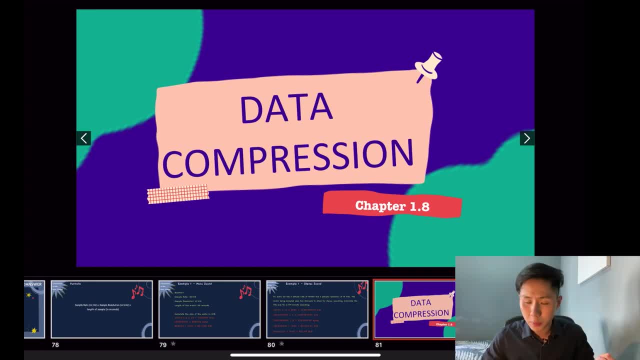 we need to increase the color depth, the sampling resolution, which would result in an increase in size, And there is a way that we can compress all this file so that we can retain the information, but losing some of the storage size. So let's see how we can do this. 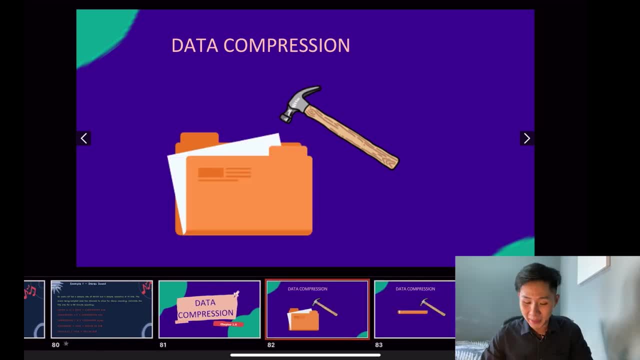 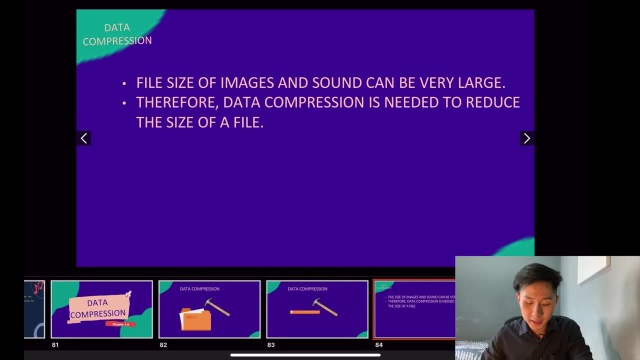 how we can compress the data, just like in this animation here, And like what I said, file size of images and sound can be very large. Therefore, we need to do something called data compression. It is equivalent to the zip function in your computer. 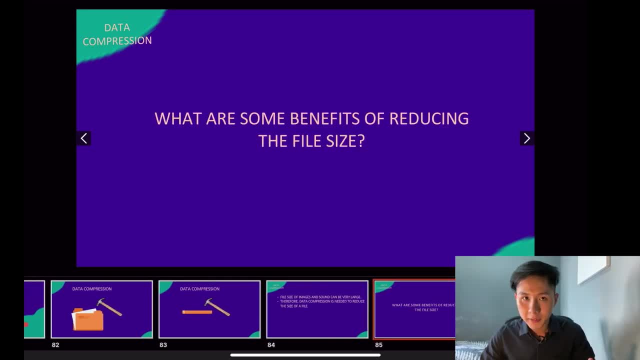 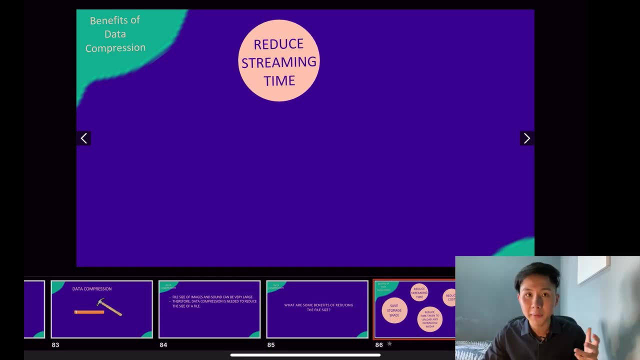 if you noticed. So here are some of the benefits to reduce the file size. The first thing is that we can reduce the streaming time, which means if this video size is smaller, it is easier for me to upload it to YouTube And reduce time taken to upload and download media. 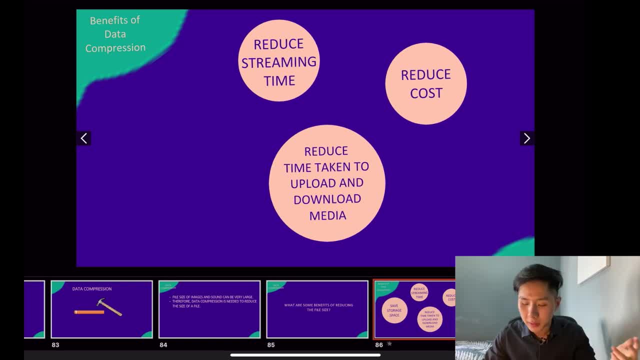 reduce cost. Cost is very important. If you go to the market and try to look for a 128 gigabytes and 256 GB of hard disk, you will know that the price is very different. Therefore, by reducing the size, we can actually reduce the cost. 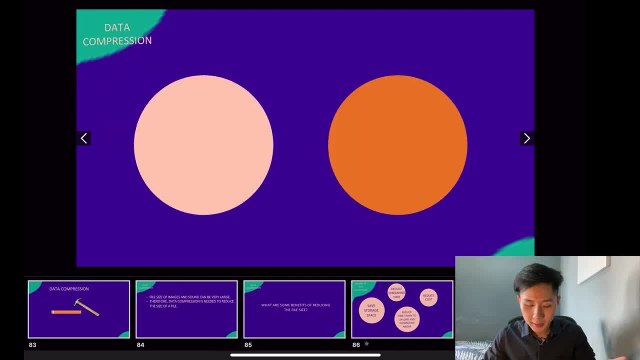 and save storage space very straightforward. So there are two different types of data compression that can be carried out for what we will learn in our syllabus. The first one is called the lossy file expression compression- file compression. Second one is called the lossless file compression. 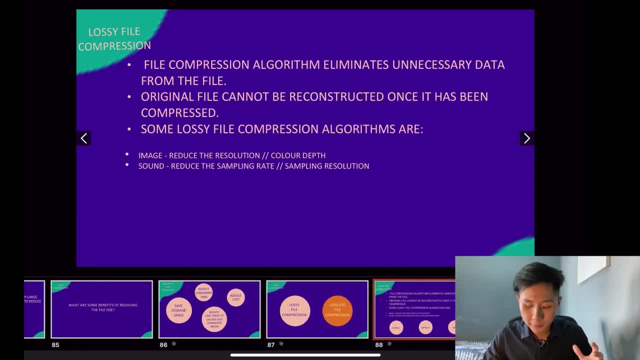 So let's start off with the lossy file compression. It is an algorithm that eliminates unnecessary data from the file, And one setback of it is that the original file, once you have compressed it, it cannot be reconstructed. And some of the lossy file compression algorithm. 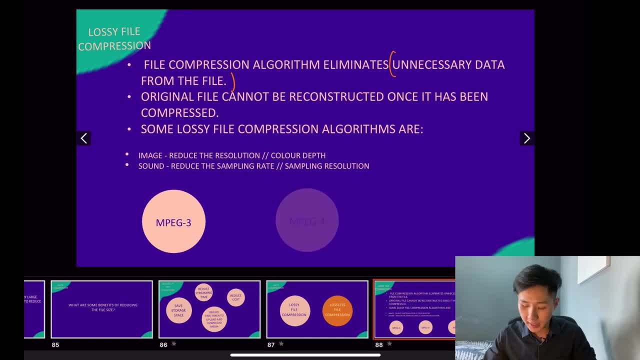 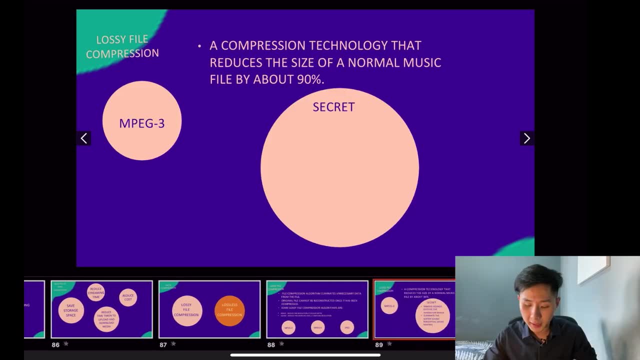 that we will learn is the MPEG-3, the MPEG-4,, MP4, and also the JPEG. So here are some of the details of MP3.. It's a compression technology that reduces the size of a normal music size, followed by 90%. 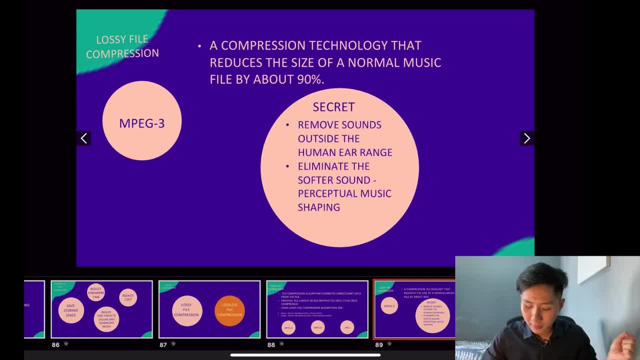 And the way that it does that is to remove sounds outside the human ear range, which means when we record a sound, there is certain sound that cannot be heard by us, but they pick up some of the storage space. So this algorithm, they remove all the sounds that we cannot hear. 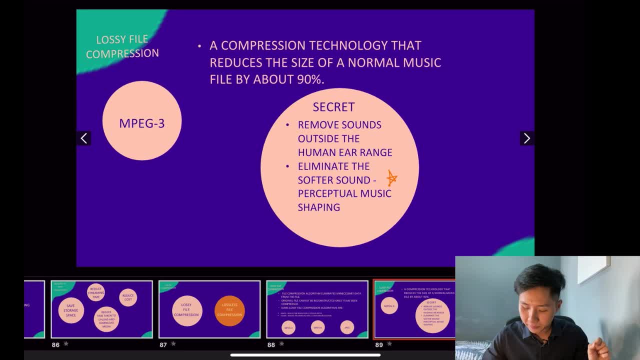 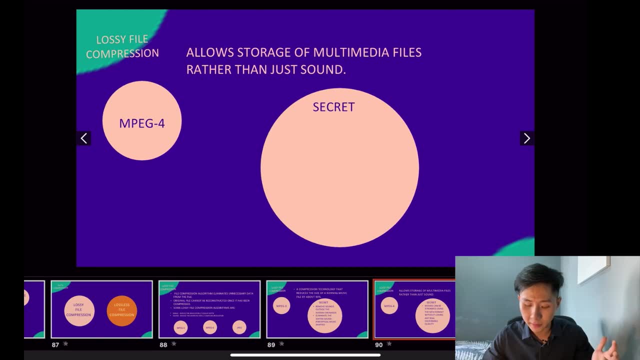 and they eliminate. look at point number two, the softer sound that we can't hear. So that's MP3.. So MP4 is a large storage of multimedia file rather than sound, And the secret of how you compress files is that it removes certain pixels in the algorithm. 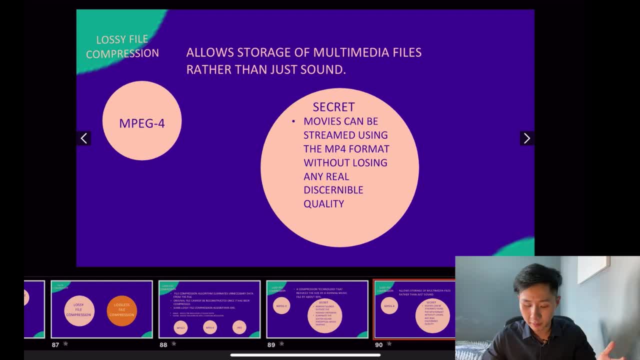 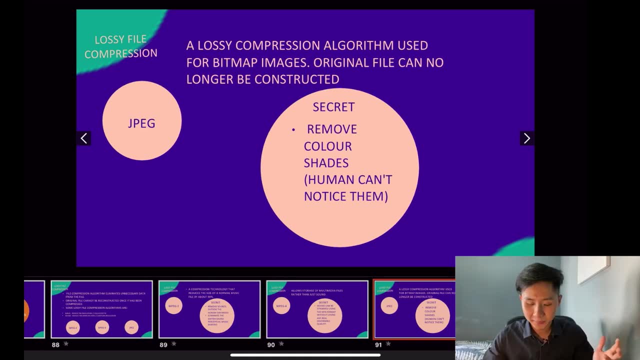 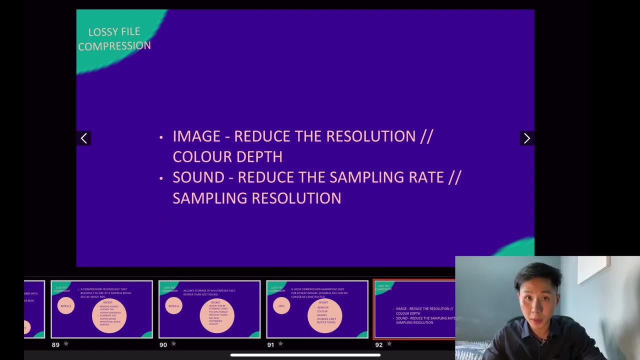 in the video without us noticing what is different. That's for video And JPEG is for the image. It will reduce color shades that we cannot notice. So this is how we reduce the size of image and sound. So, if you remember how we calculate the formula, 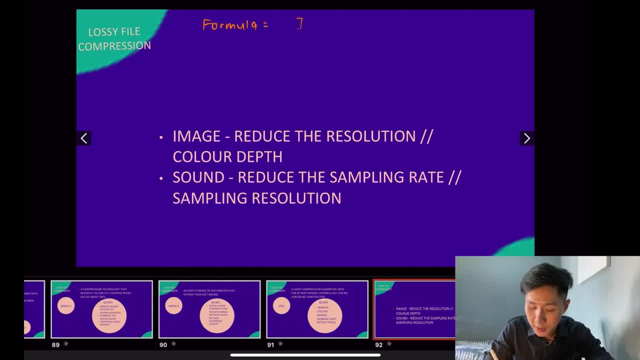 to calculate the size of image is image resolution multiplied by color depth, which then will give us the size. Therefore, if today I asked you how do we reduce the size of an image, there are literally only two methods. First of all, we reduce. 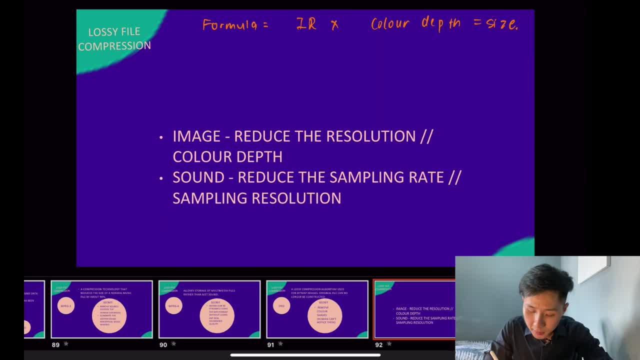 let me use another color. we reduce the image resolution or we reduce the color depth of the image. So that's how we can do this. This is- I think I believe it's- a PASA exam question. They said: how does lossy file compression reduce the size of an image? 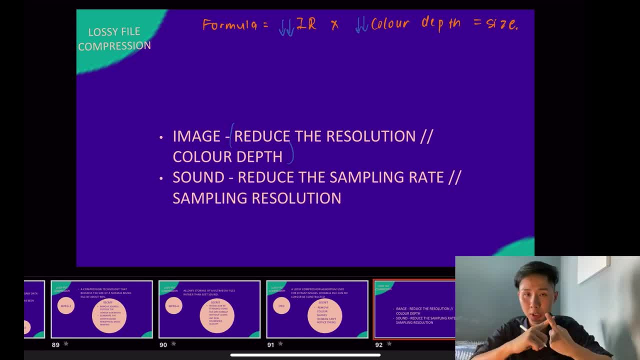 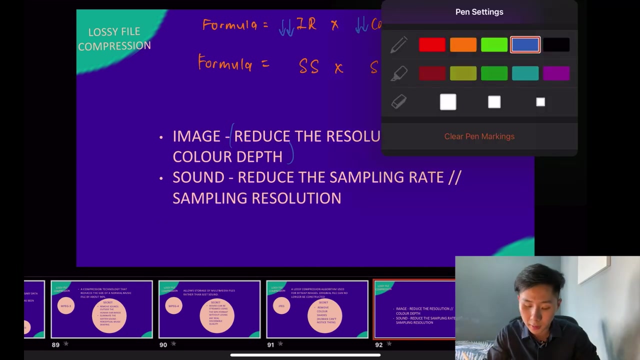 So that's the two methods that you can use: Reduce the resolution, Reduce the color depth, And another. let's move on to the formula to calculate a sound, which is sample rate multiplied by sampling, resolution multiplied by time. So the way we can reduce the file size of a sound. 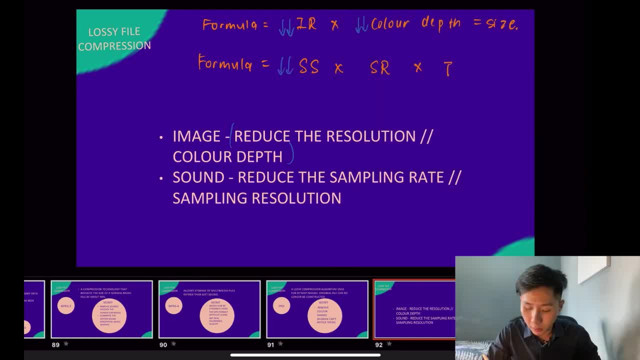 again is: either we reduce the sample rate, or we reduce the sampling resolution, or we can even reduce the length of the video. So that's how all these things can be linked together. So, having talked about lossy file compression, the way that I remember this type of file compression- 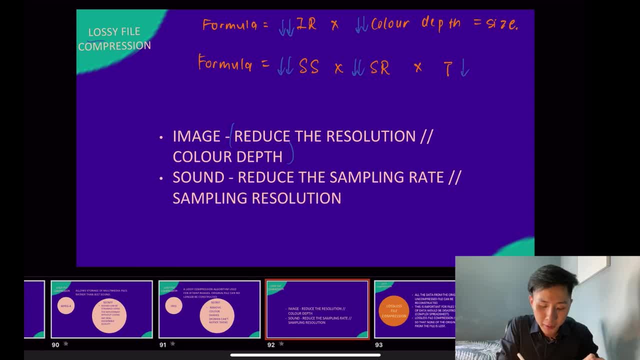 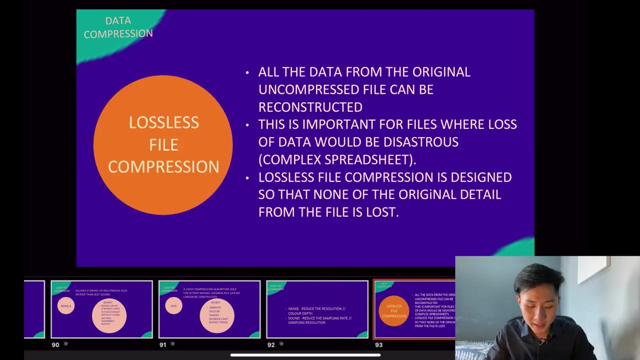 is that instead of lossy, I call it lousy, because once the file size is being compressed, once the file is being compressed, it cannot be reconstructed. It is very lousy. But here's another data compression method which is better than lossy compression. 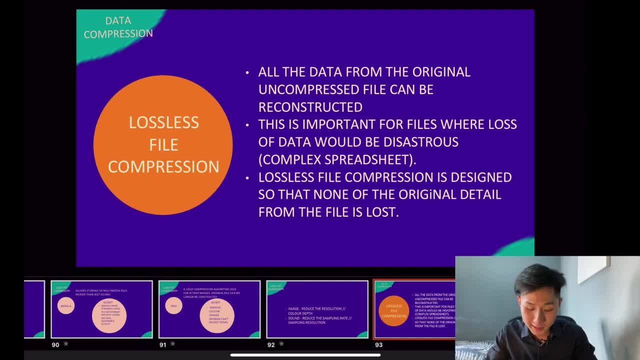 Which is called the lossless file compression, As implied by the name. once you compress it, you won't lose any forms of data. It's lossless, You won't lose any. And what they say here? all the data from the original, uncompressed file. 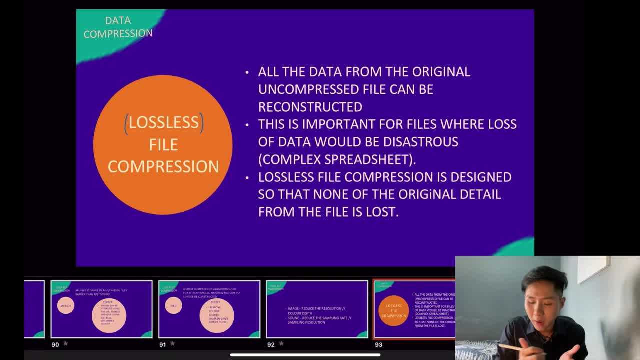 can be reconstructed Once you compress it from. let's say you have a file, you compress it- see F compressed file. you can reconstruct it back to F. This is important because sometimes when we compress file, we don't want to lose out some important information. 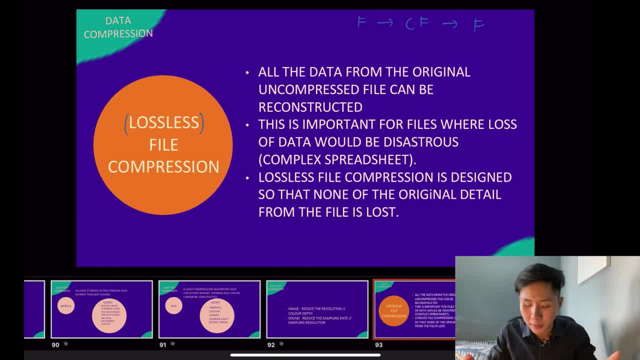 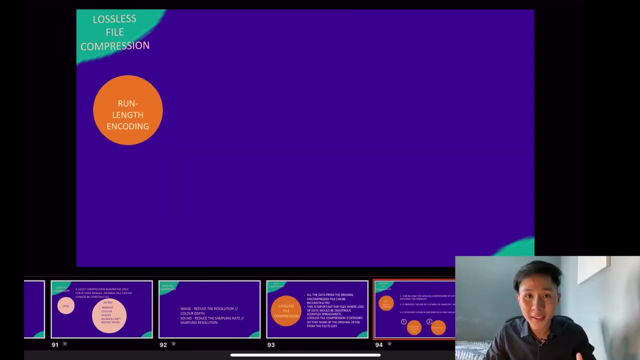 such as: let's say, you are working on a very complex spreadsheet for your company. you don't want to lose certain data. It is a compression algorithm that is designed so that none of the original details from the file is lost. So one type of algorithm that do lossless file compression. 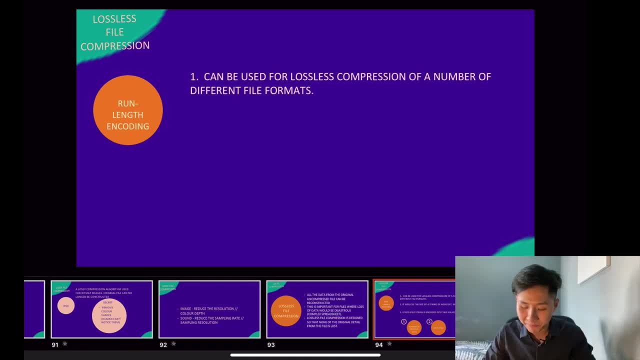 is called a run length encoding. So what it does is that it is used for a compression of numbers of different file formats. It reduces the size of a string of adjacent- that's the keyword- and identical data. A repeated string is encoded into two values. 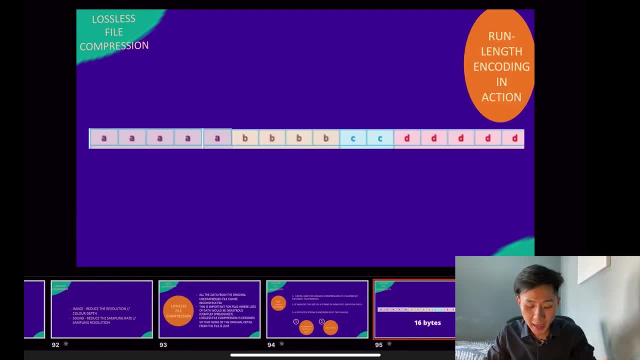 Let me give you an example here. Let's say, we have the data here, We have five A's, four B, two C, five D concatenated together And they are just identical of each other and they are adjacent of each other. 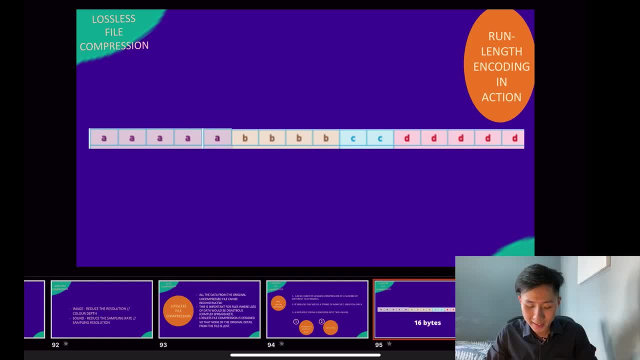 And how run length encoding would do, is that? so the file size here would be 16 bytes, assuming that each character is represented by 8 bits. But there's a way for us to further compress this file. So let's say we can actually encode.